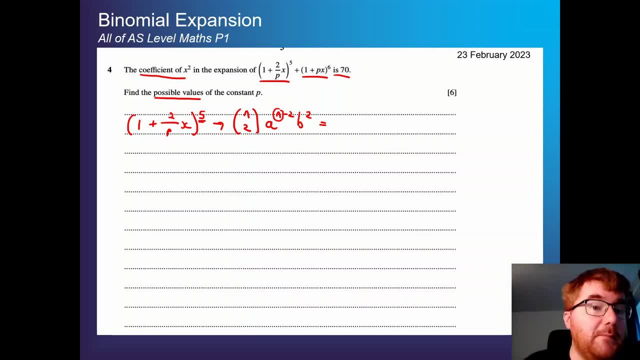 where's the 5 come from? This n comes from the total power for the bracket. So we can then work out: then 5,, 2,, like so, and then a cubed, because n is 5 here, and then the b squared. Now we just 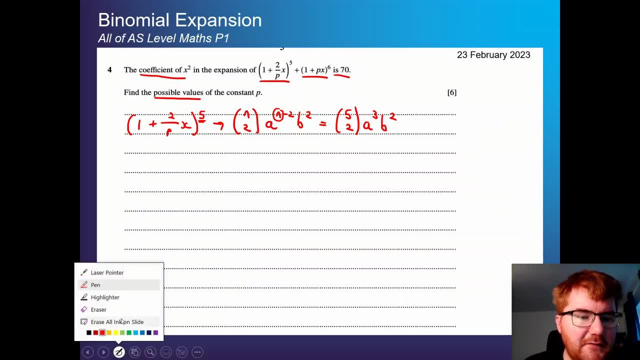 need to substitute in the x squared term. So we're going to take n here and we're going to take the b squared term. So, if I highlight this, this first term is going to be a- Let me just make that nice and clear- And this is going to be our b. Now we're going to do a lot of questions on this in. 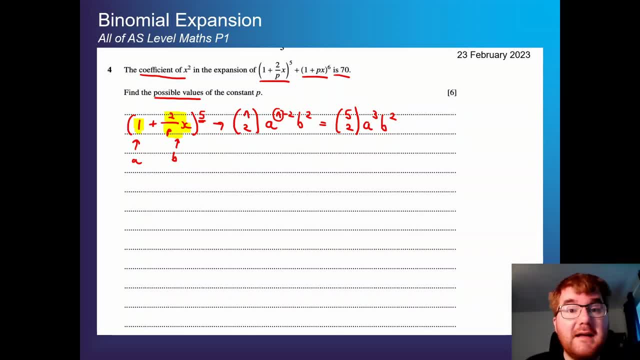 this video. So if you're not so sure at the moment, then don't worry, we'll be getting lots and lots of practice. So what this will do, then we'll get 5.. We tend to call this choose 2.. So 5, choose 2.. 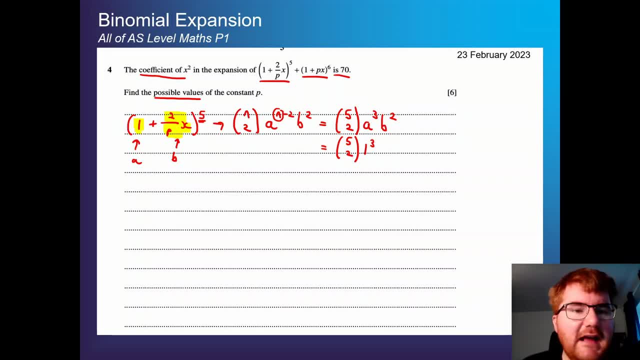 a is 1, so it's 1,, which is going to be 1, and then b squared, So 2 over p, x squared. Now you're probably looking at this bracket thing. It looks like a vector, doesn't it? And exactly how we work this out. Now we don't. 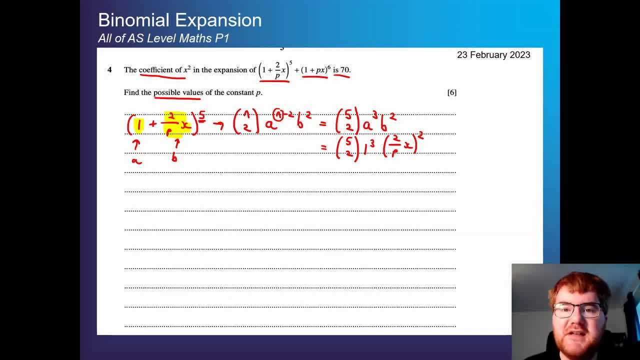 have to do this manually. This is where the calculator comes in. Now, on the calculator, they tend to write this slightly differently. They tend to write this as 5, choose 2, hence this c in the middle. But notice notation. 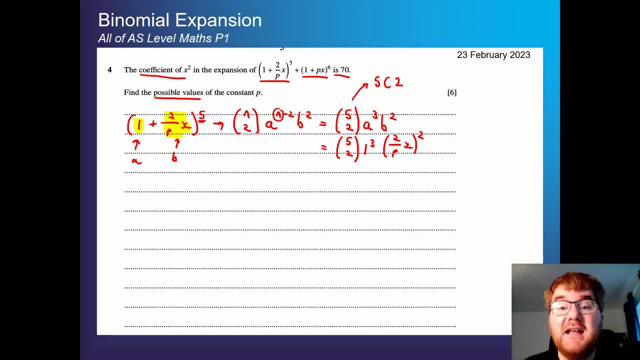 You'll see this in the formula booklet, but also in the mark schemes They tend to use this big bracket notation, and I tend to use that on most courses as well. So what we're going to do is work out what this 5 choose 2 is by using the calculator. So make sure you've got your calculator. 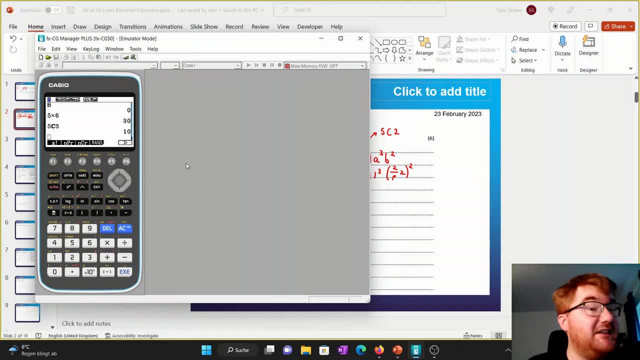 set up. I'm going to be using the CG50 here. We've got a class whiz. Actually, in some ways it's easier. You're going to be looking for a yellow part on the button which has a c, So I'm going to. 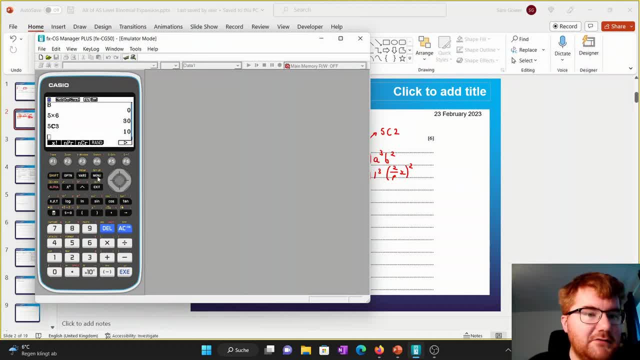 use this calculator here. So I'm going to use this calculator here, And then I'm going to put this in the calculator. So what we're going to do is we're going to use this calculator here, And this is the same calculator we used to use for our last class. So this is the calculator We're going to use this. 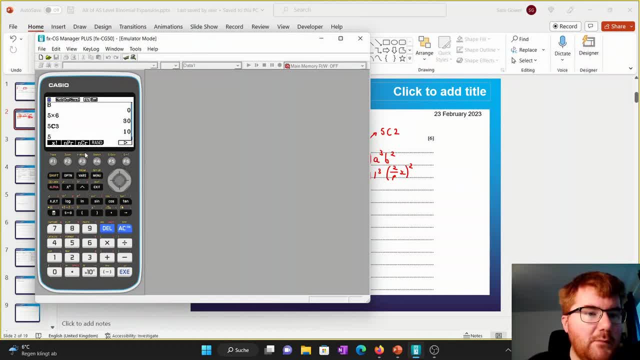 calculator here, And if you click on this button, you can see that we've got this ncr selected already. If you're wondering where this comes from, you go to Options, you press F6 to go to Probability and then the functions will appear. And we want to do 5 choose 2.. So all we have to do here is click on 5.. We click on F3 to give us the c button, And then 2.. And that will generate then 10.. So we're going to be using 5 choose 2, which is 10.. So all I'm going to do is, wherever I see a 5 choose 2,, I'm going to put 8.. 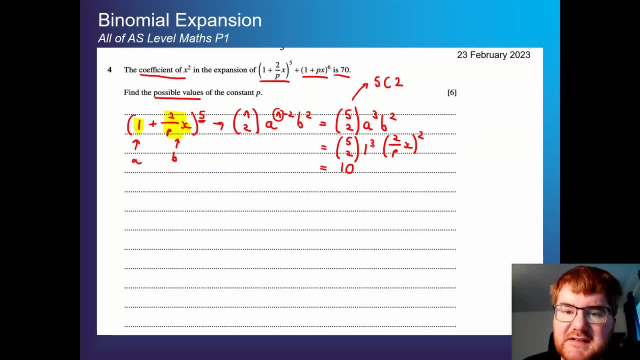 10. 1 and anything times by 1 just stays the same, and then we're going to get 2 over p, x all squared. This is where we have to be quite careful, remember. it's squaring the entire thing. so we get 10 times or. 2 squared is equal to 4, p squared is just p squared, and then x squared is: 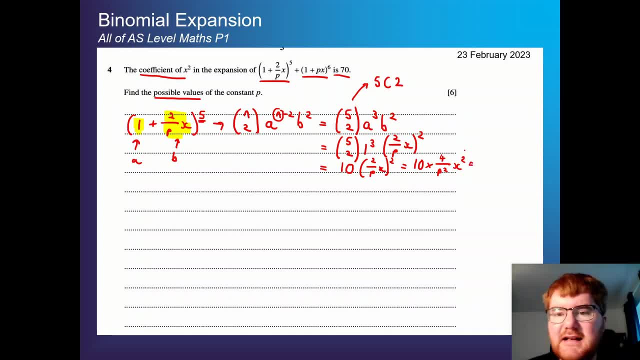 just x squared and we can tidy this up slightly. so 10 times 4 is equal to 40, so we get 40 over p squared, x squared. So we've managed to work out the x squared term of that first bracket and we're going to consider- let's highlight this, we're going to be considering that coefficient. 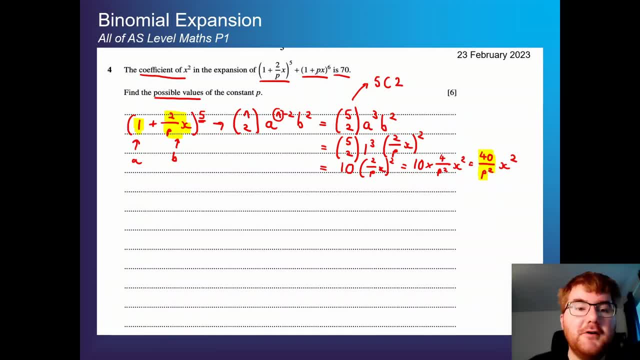 a little bit later on. Now let's do exactly the same process. we're going to get some good practice here of 1 plus p x to the power of 6. so we get 1 plus px to the power of 6. so let's have a look at which term that we want. remember, we want the x. 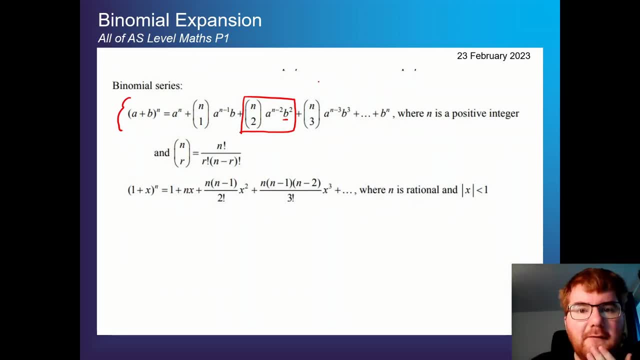 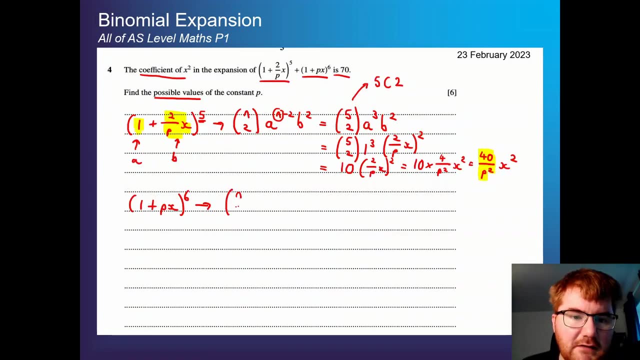 squared term. so we go back to our formula sheets. we want to use the same thing in the box here as we did before, so I'm just going to write that down. so n 2 a, n minus 2 b squared- okay, but this we have to be slightly careful because, notice, our power here is now 6, it's not 5. so then we're going. 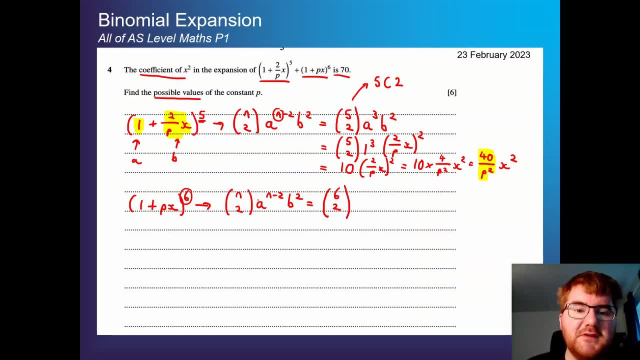 to do 6, choose 2, which we'll work out in a moment. we're going to do a to the power of 4, remember 6 minus 2 is 4 and then b squared. so if we work this out, let's just do 6, choose 2. nice and quickly. 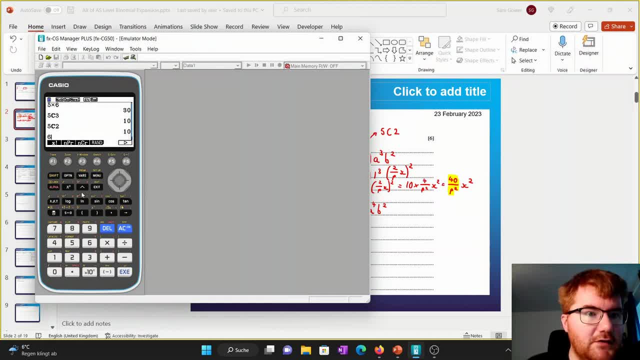 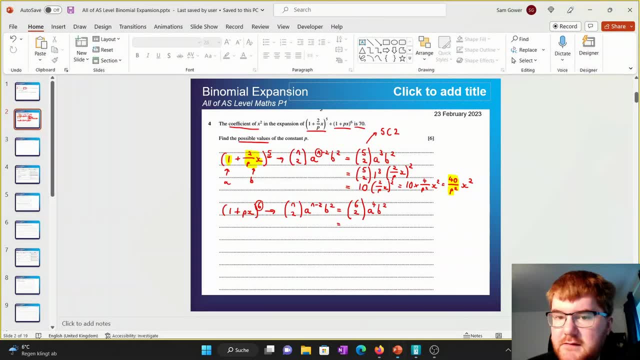 okay, so we just type in 6, choose 2, and that's going to generate us 15, so we can replace that with 15. now we're going to get 1 to the power of 4, and then we're going to do 6, choose 2, and then 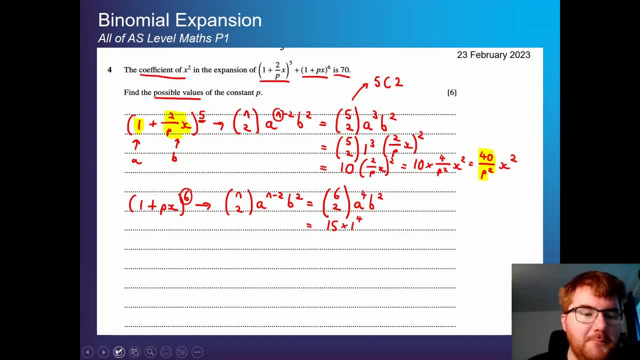 we're going to get 1 to the power of 4, again our a term, just like we did before. let me just highlight this again. I'll go more quickly through the subsequent questions. but yeah, this is going to be our a, this is going to be our b. so you get 1 to the power of 4 and then we're going to get 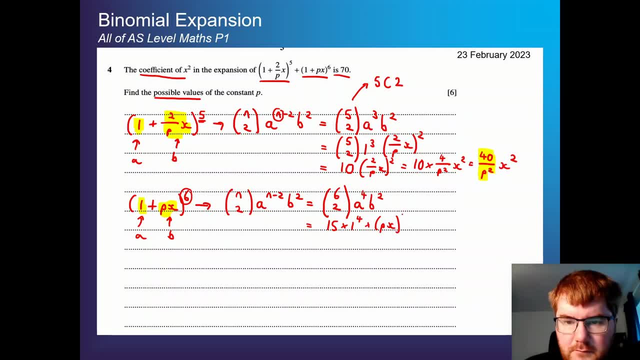 this squared, so we're going to get px all squared. now we can do a little bit of tidying up here. so 15 is fine. 1. power 4 is just 1. p squared is just p squared. so we're going to do a little bit of. 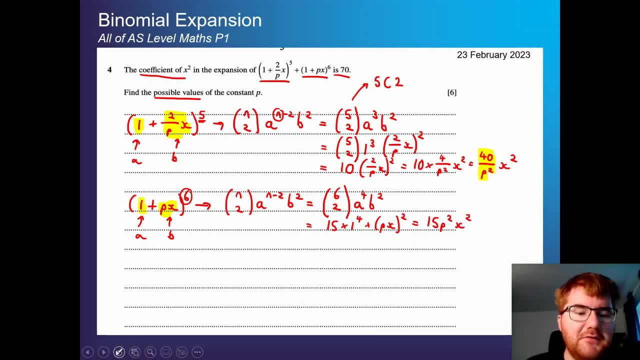 tidying up here with x squared. now, leadership went off the Flynn correlation and said: this p is also over there and if we add 2 to the power of 5, which I've calculated now is 2, we're going to have p squared as 9–4 plus 3. so this is going to be baby p squared in my. So we've got k squared. 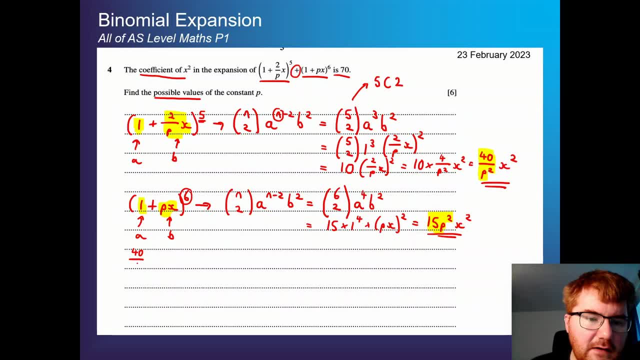 we've got to add in delta, as I mentioned earlier. so let's just solve this Pointa sacred well, you and then add together 15p squared x squared. what that's saying is going to be equal to 70x squared, and in order for that to be true, then that means that this plus this, the coefficients. 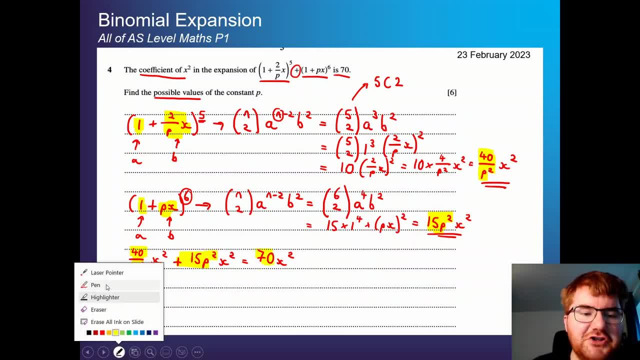 must be equal to this. so this allows us to generate an equation to try and solve for p. so we get 40 over p squared plus 15. p squared is equal to 70, and this is where the quadratics come really, really useful. i've done a video on this as well, so do check that out in the description: 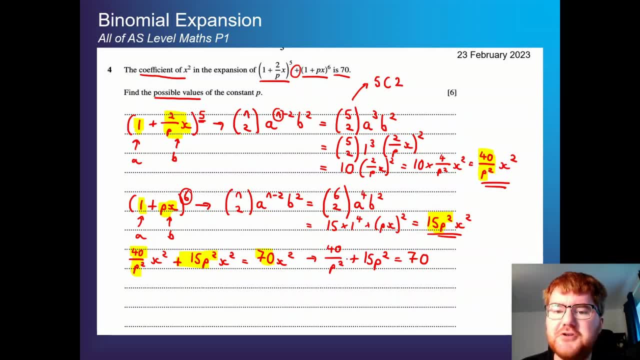 and we now need to solve this. so the general approach here is that we don't really don't like fractions, so we don't like fractions, let's get rid of it. so what's the opposite of dividing by p squared? well, that's times by p squared. 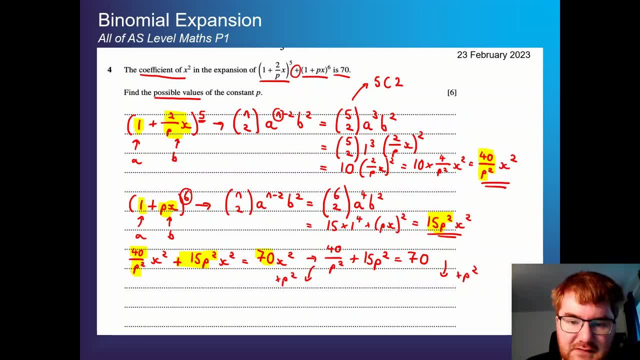 so we get 40 over p squared plus 15p squared is equal to 70, and this is where the quadratics come really, really useful. i've done a video on this as well, so do check that out in the description on all sides of the equation. so this cancels, give us just 40, 15p squared times. p squared is 15. 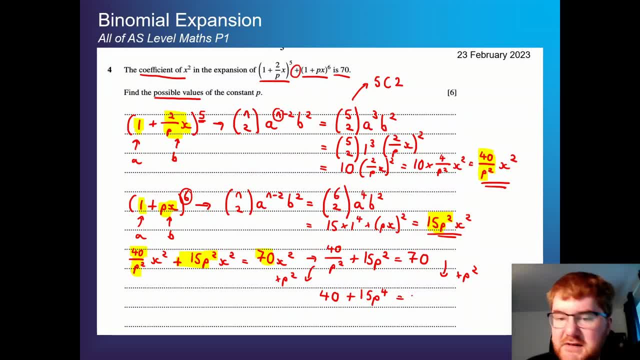 to the power of 4 and then 70 times p squared is just 70p squared. so we've now got an equation that we can work with this: 40 plus 15p to power of 4 or 70p squared. i'm just going to write it. 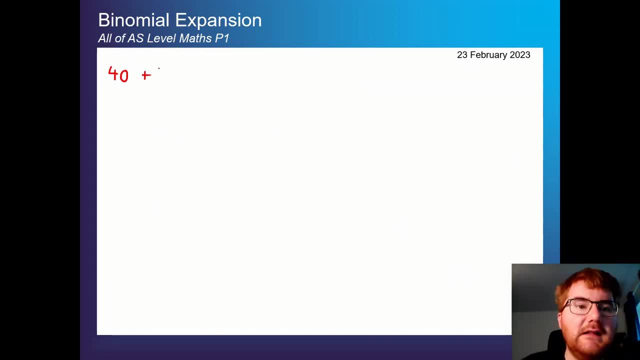 on this slide here, so 40. so we've got a little bit more space to work with this now. at the moment, um, it looks like something we can't solve because we've got a quartic, but we can make this look like something that we are familiar with now. a general approach. 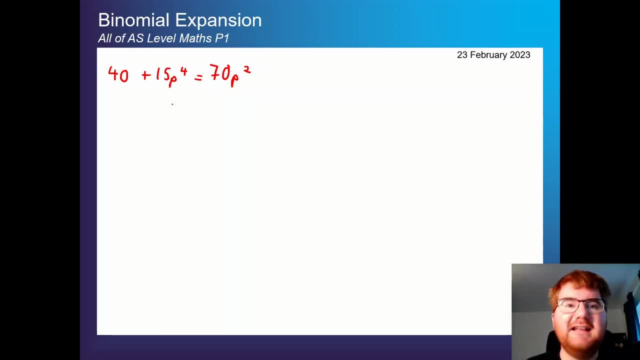 when you're working with cubics or you're working with quadratics or anything is, make sure you get the right hand side zero. so we're going to do that by minusing 70p squared on both sides. if we do that, i'm going to move this around slightly, so 15p. 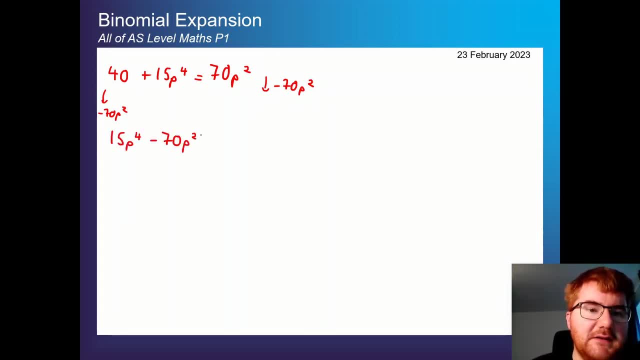 to power of 4 minus 70p, squared plus 40 is equal to zero notice. there is a common factor here as well, so we can actually divide through by 5. again, we want to try and make this as easy to deal with as possible. we divide 3 by 5. 15 divided by 5 is 3. so 3 to p to power of 4, and if we divide this by: 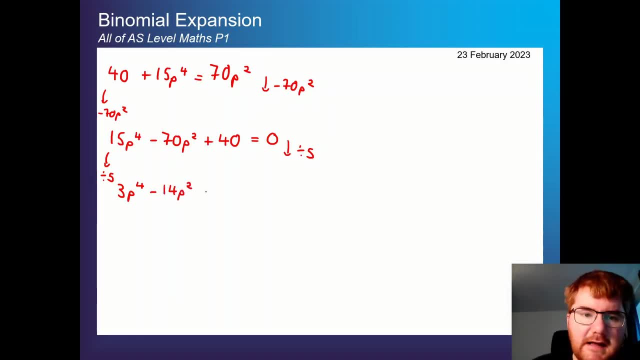 5, we get 14, so 14p squared. and then we divide this by 5 and we get 14p squared, and then we get 14p squared, and then plus 10 is equal to zero. now you can go directly to actually factorizing this. 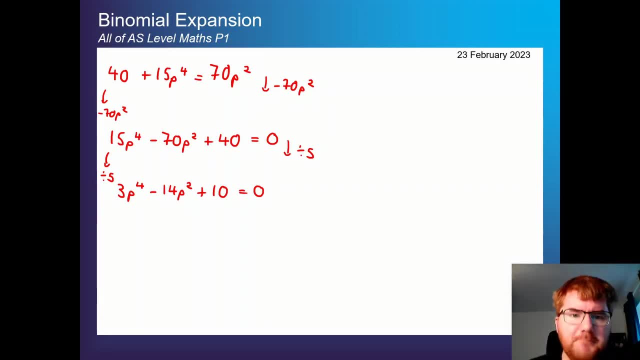 if you're comfortable with that. if you're not so comfortable, then we can do a very quick substitution. so i'm going to let: u is equal to p squared, and if i square both sides, that means then that u squared is equal to p squared, all squared, which is equal to p to power of 4. by doing this i 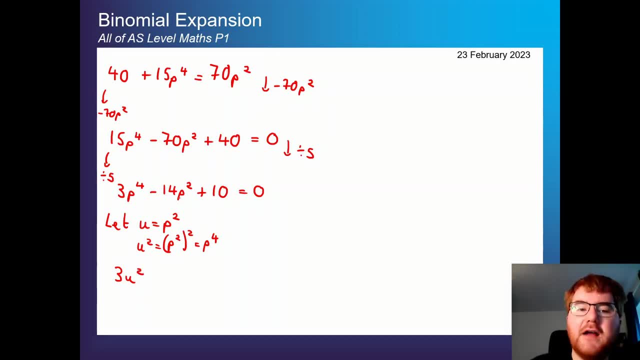 get 3u squared, i can replace the p squared with just u and notice we get a quadratic that we can actually go about solving. now the way i generally teach this factorizing technique is: i set up my brackets and we kind of work with a trial and error approach. it's usually quicker and, as you, 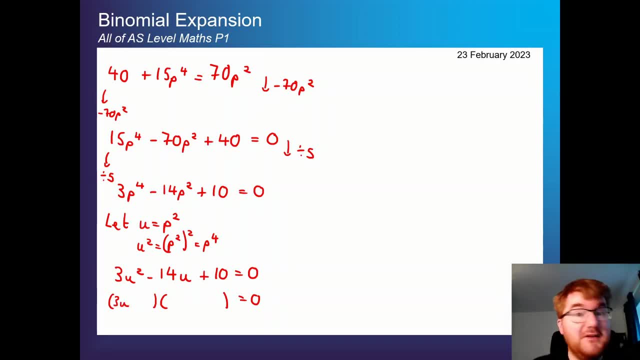 go through the a level maths course, you're going to need these quick methods to get these easy marks. so first of all, put 3u and u, because the only way we can time something together to give us 3u and u is by doing this. so we're going to do a quick method to get these easy marks. 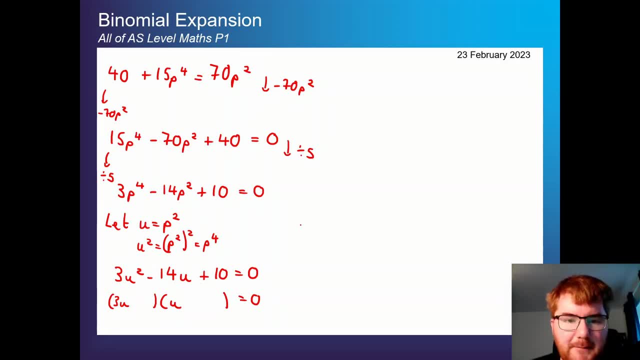 3u squared, and now we need to decide what numbers to put in here. well, the factors of 10 here are 1 and 10 and 2 and 5. again, we can have negatives and positives as well. looking at this, this is 10. 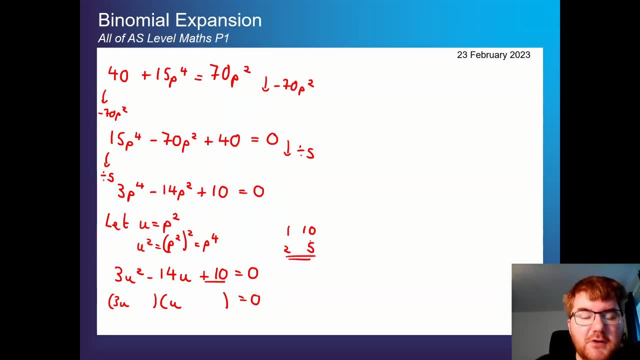 and 14 are quite close to each other, so i'm going to be tending towards the 2 and 5, and now we can have a look and see what we want to put in at this point. so with this here, seeing if there's anything. 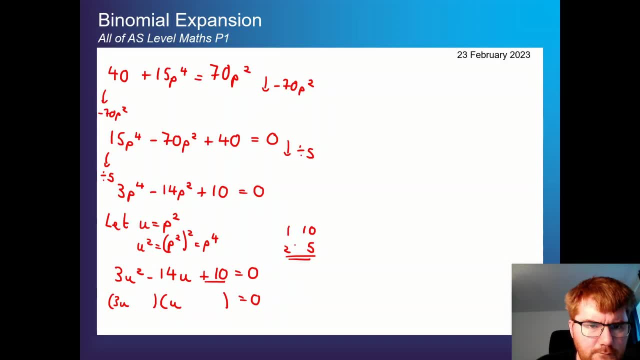 that's sticking out immediately and there isn't again. i'm just going to be checking signs here to make sure that we've done everything correctly. and again, this is the key technique. when you're looking through this, this is not factorizing correctly. so i'm looking back through my working and the next thing i 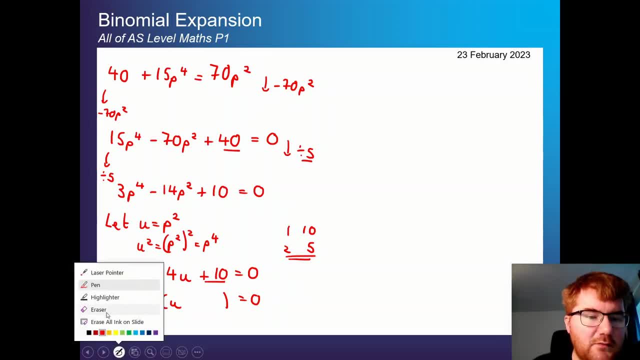 notice is that 40 divided by 5 is not 10, it's equal to 8. so i'm leaving this in the video on purpose, so you can see. even if it doesn't go exactly as you expect it doesn't factor ize nicely, then the best thing you should do is go and check your working and then see if there's. 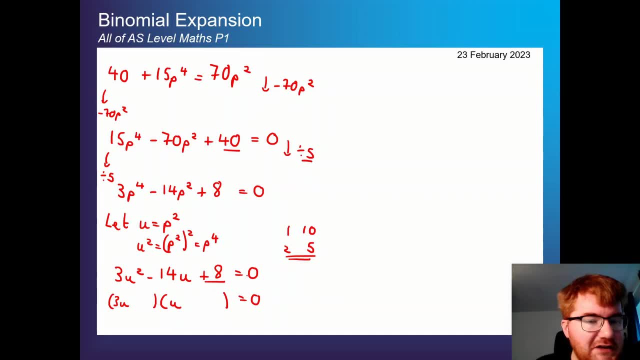 something you can correct. so it should actually be plus 8 here. so again, we're going to change our factors then to everything that multiplies to give us 8. that's going to be 1 and 8 and 2 and 4- again pluses and minuses, and at this point, yes, there is something that works- we get a minus 4. 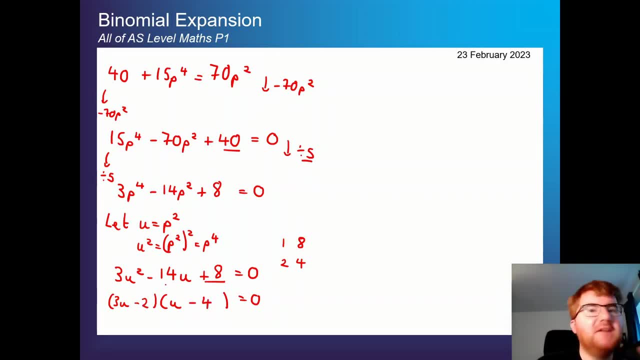 here we get a minus 2 here. now, how am i supposed to do this? well, i'm going to be checking the results of this so quickly. well, what i'm doing my head here, essentially, is just multiplying the cross terms. so, minus 4 times 3u is minus 12u. minus 2 times u is minus 2u. minus 12u minus 2u is minus. 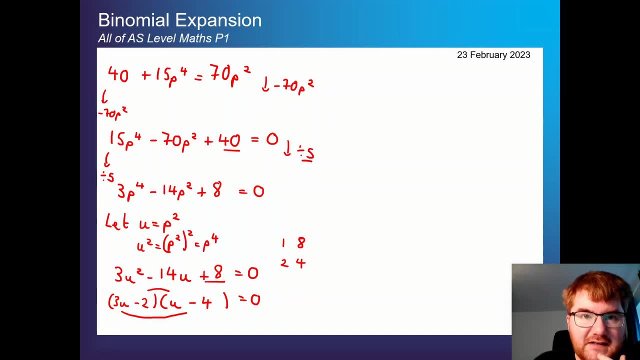 14u, so we do get our correct factorization. i really encourage you to use this kind of method. it will make your work a bit easier now. if we solve this well, that means then either that 3u minus 2 is equal to 0, so u is equal to two thirds. 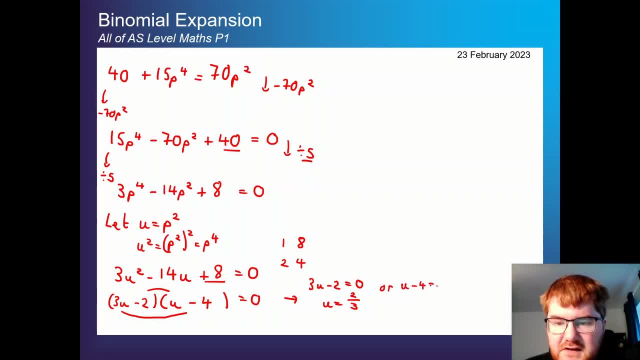 or u minus 4 is 0, so u is equal to 4. again, we're not quite solved at this point because, remember, we used a substitution, so we're going to do a back substitution at this point. that means, then, that p squared is equal to two thirds and p squared is equal to 4, and now we just need to. 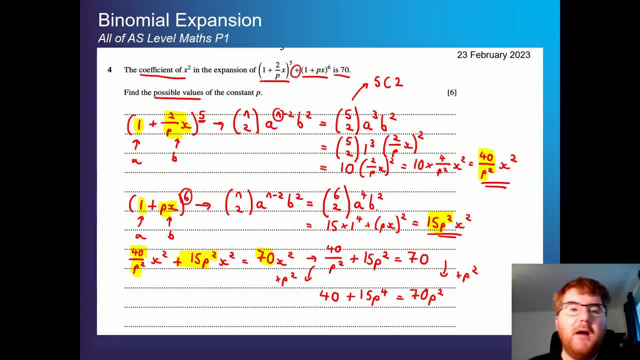 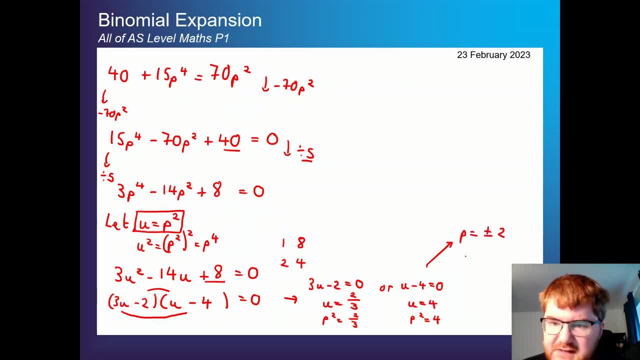 minus 4 and we're going to get a plus minus 2, which comes from this answer. don't forget plus minus. and we also get the plus minus the square root of the fractions. so those are our four answers. there p equals plus minus 2 and then p is equal to plus minus root 2 over 3. make sure it's nice. 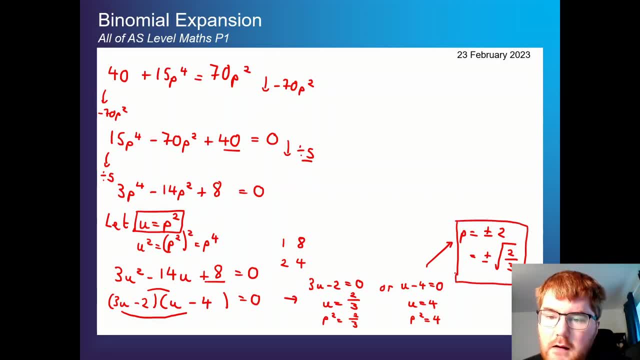 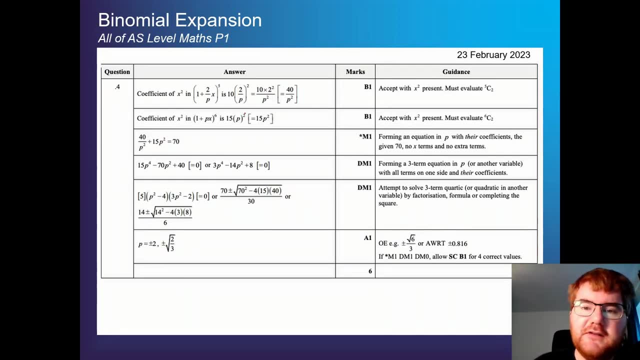 and clear for the examiner so they can see exactly where those four answers are. okay, and you can check your working here so you can see all the different steps i've gone through. notice: if you're not happy with the factorizing process, you could have always used a quadratic formula as well. that is also a perfectly valid method to get to these. 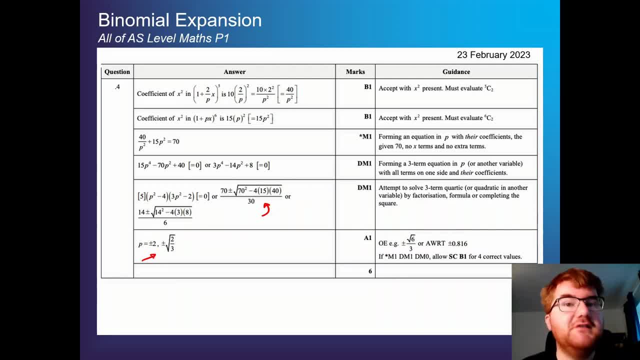 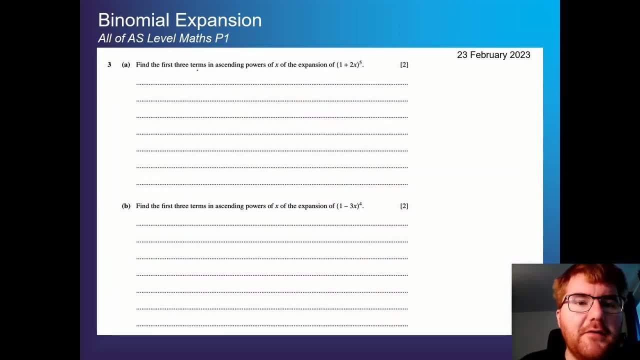 four answers at the bottom: plus minus 2 and plus minus root 2 over 3. okay, and on to the next question. so find the first three terms in ascending powers of x, so essentially the powers going upwards. okay, so you start with your constant term, then the x term, then the x squared term and then the x cubed term, if appropriate. 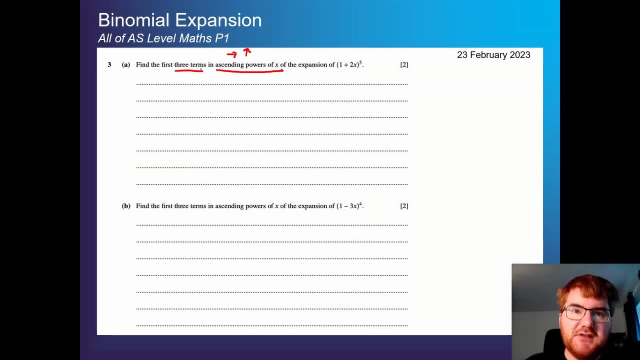 notice, we're looking for the first three terms, so it's going to be a constant term, an x term and an x squared term. so let's go with 1 plus 2x to the power of 5, and this is a case of just using your. 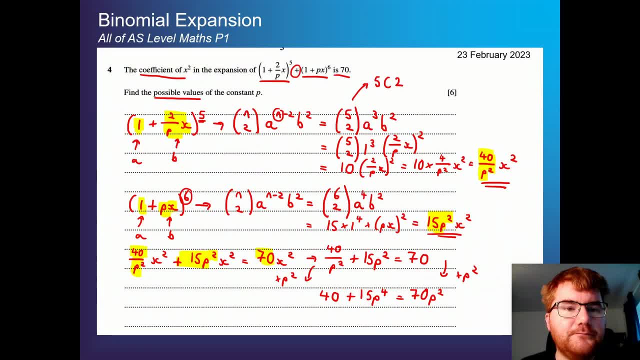 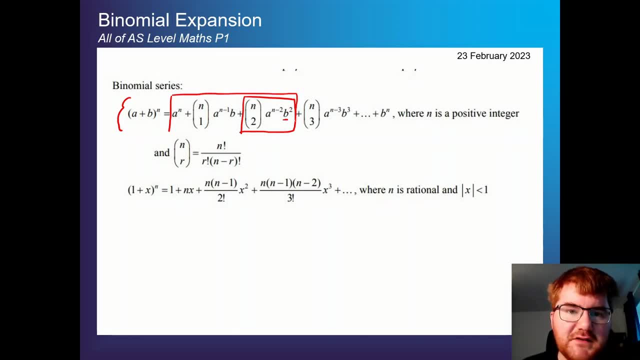 formula sheet nice and carefully. so if we go back we're going to be using this formula sheet here and we want to go for the first three terms, so we want this part here. so the eighth power of n plus n. choose 1 a n to the power of n minus 1 b. 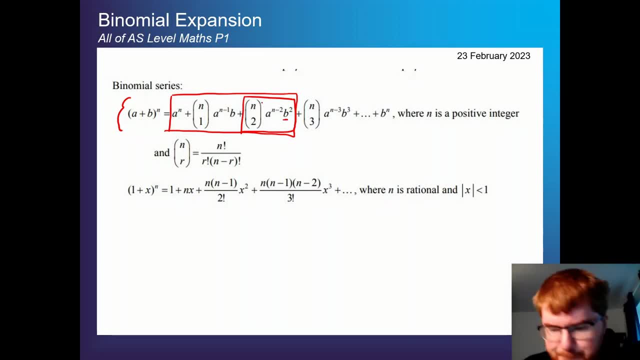 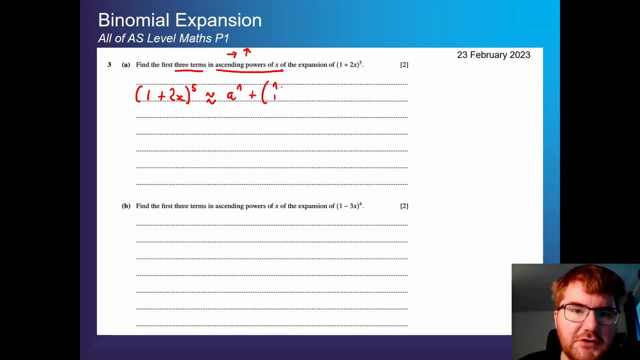 plus n, choose 2 a. power of n minus 2 b squared. so i'm just going to copy that across, just so that we've got that there and choose 1 a to the power of n minus 1 b. again, there's no harm in writing extra working, particularly if you're starting out with this. 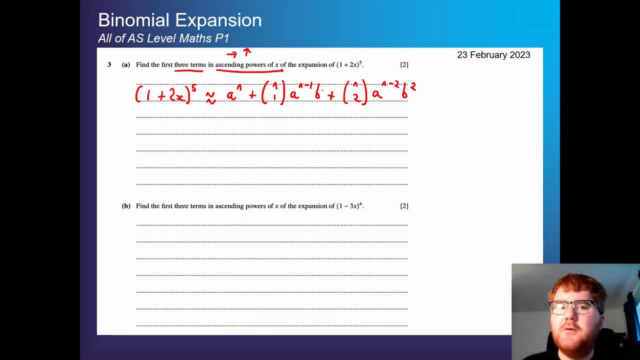 kind of topic. this is quite a useful thing to do. i just want three terms, so i don't need to write any more than that. now, remember our a and b. let's identify that first of all. so we've got our a, which is going to be 1 here, and then b, it's going to be 2x, and then our n- it's going to be. 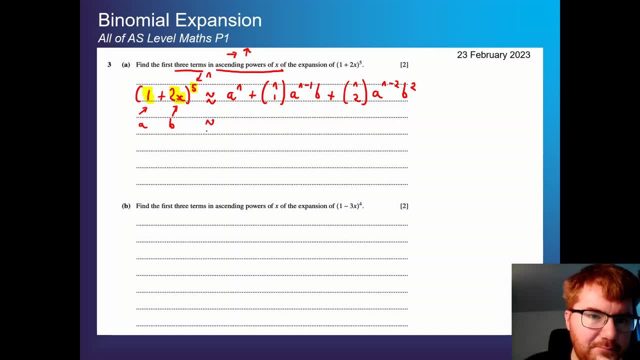 that total power, which is 5. so if we expand this out, we get 1 to the power of 5. that's just 1, and then we're going to get 5. choose 1, which will work out a bit later on. again, we always get 1s. 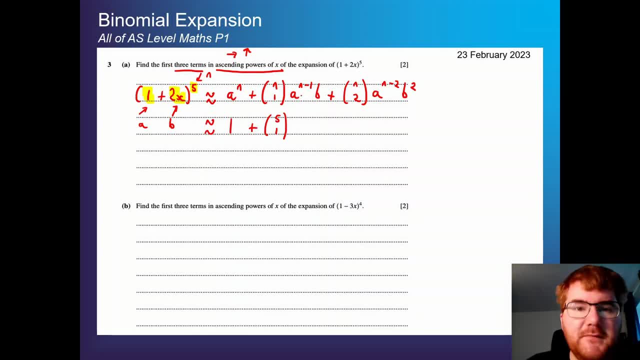 essentially for these a terms. so we can kind of ignore them, because 1 to the power of anything is just 1. so we're going to get b first of all, which is 2x, and then we're going to have 5- choose 2 again. the a term is just going to stay as 1, and then we get 2x all squared. now, this is really. 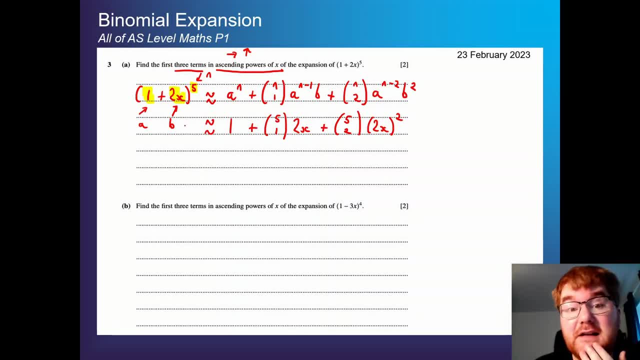 important making sure you're squaring the entire 2x term. at this point we just need to work out the 5 choose 1 and 5 choose 2. we could use the formula from the formula sheet. let's get used to using that calculator, okay. well, we already worked out 5 choose 2 from the previous question, but let's 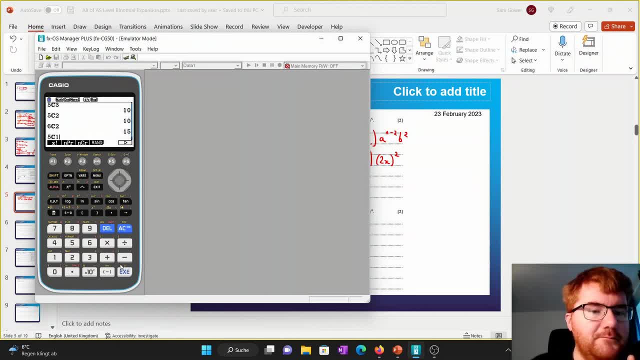 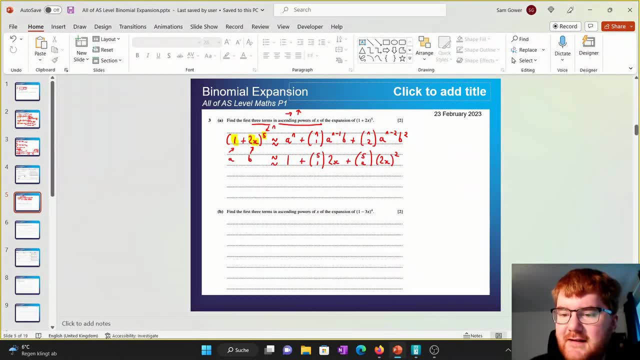 just work out quickly: 5 choose 1. this is going to be equal to 5, so we've got 5 and 10 for those two binomial coefficients. so we get 1 plus well, 5 times 2 is just 10, so we get 10x. 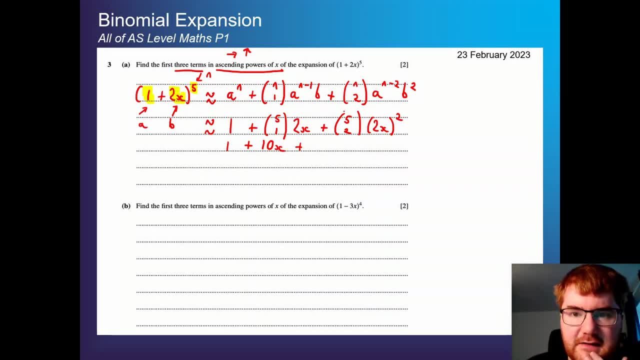 and 5. choose 2 is just 10, so we get 10x and 5 choose 2 is just 10, so we get 10x. and 5 choose 2 is equal to 10, so we get 10 times. now this is where to be really careful when the squared applies to. 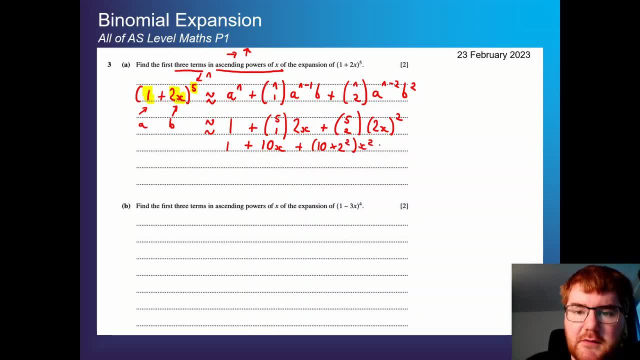 both. so we get 2 squared x squared and then this becomes 1 plus 10x plus 40x squared like. so we're going to need that a bit later on, so it's going to underline it. so we've got that for later and 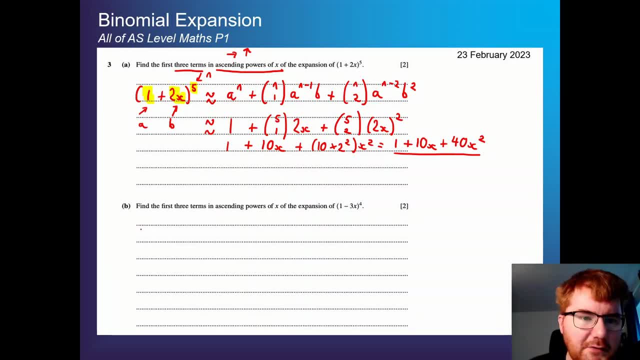 now we're going to do exactly the same process for this one here. so we've got 1 minus 3x. so we're going to be careful that minus one thing to watch out for. notice, you've got a new power here to the power of 4, hopefully getting the hang of this as we're going along. so first we're going to 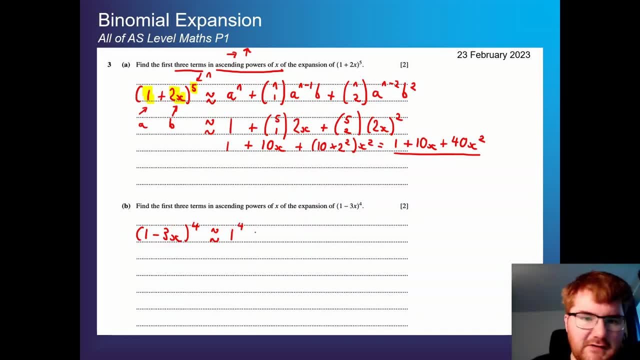 have 1 to the power of 4. it's going to be really easy to work out. now we're going to have 4 choose 1, so using that power here, 4 choose 1, 1 to power of 3 and then b, which is just minus 3x. 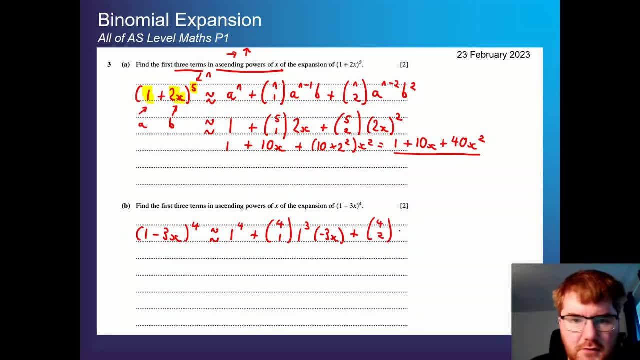 and then we've got 4 choose 2, 1 squared again, don't need to put that in- and this way, if you're really careful, minus 3x, all squared. that's really important. so, in order to work out the next part, we just need to work out 4 choose 1 and 4 choose 2, so we get 1 now. 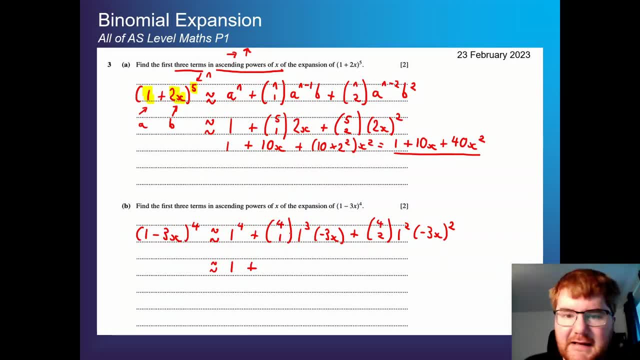 4 choose 1 is just equal to 4. you can check that on your calculator. 4 times minus 3 is minus 12. so let's move the plus there and pop in minus 12x. and now, if we just do 4 choose 2, so I've 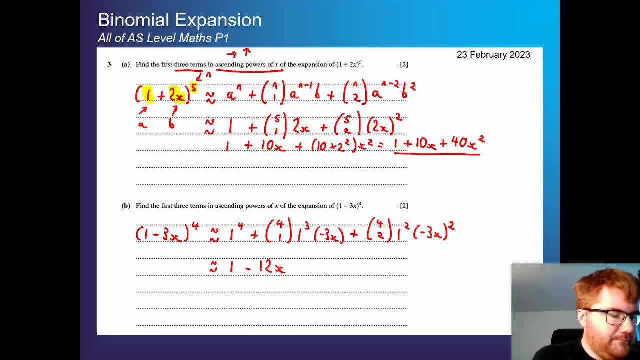 got a calculator here, so we go 4 choose is equal to 6, so we're going to get 6. now, 1 doesn't really change anything, minus 3 squared. we have to be really, really, really careful. so minus 3 squared is equal to 9, and then we get x squared. 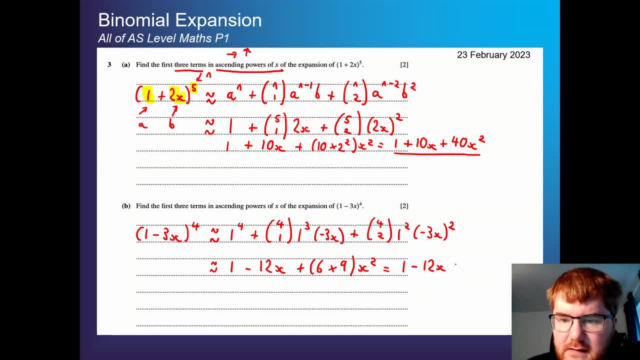 so that's going to become 1 minus 12x plus 54x squared. the biggest mistakes that are going to be made in this kind of question is that very last term and making sure that's 54x squared. okay, that's the thing to watch out for when you're doing these questions. now. very, very typical is 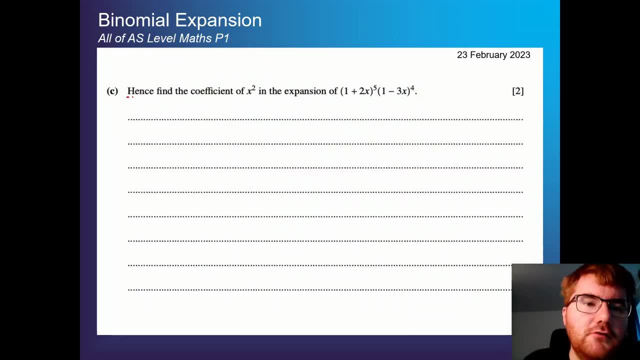 part c, which is this word hence, which often gets ignored, and it's something to really be aware of. if they use hence, you need to use parts a and b, so you need to be using what you've already done if you look at this question just separately. 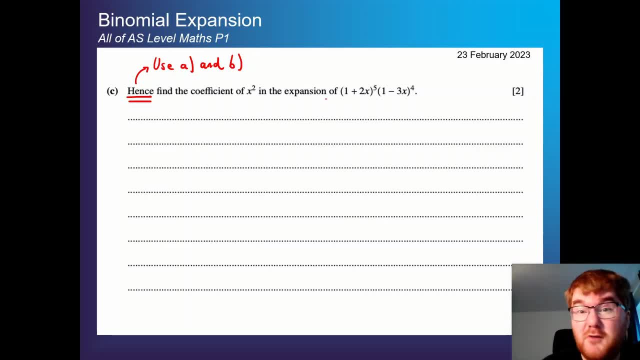 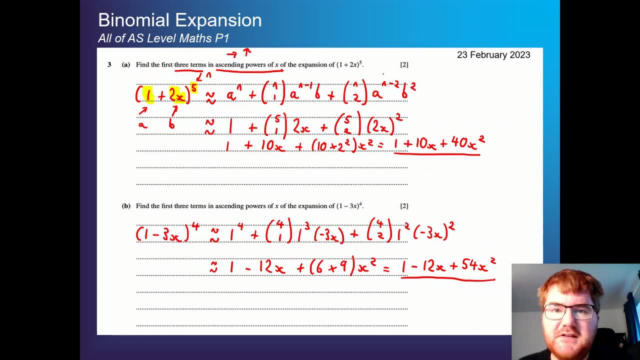 and you go find the coefficient of x squared of these two brackets multiplied, you go: oh god, okay, what's going on here? but if we're using a and b, we've already expanded these two. notice: 1 plus 2x power 5- the first bracket, and then we've got 1 minus 3x power 4, second bracket. so all I'm going. 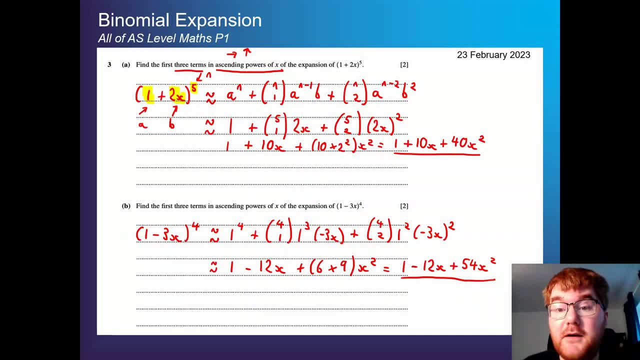 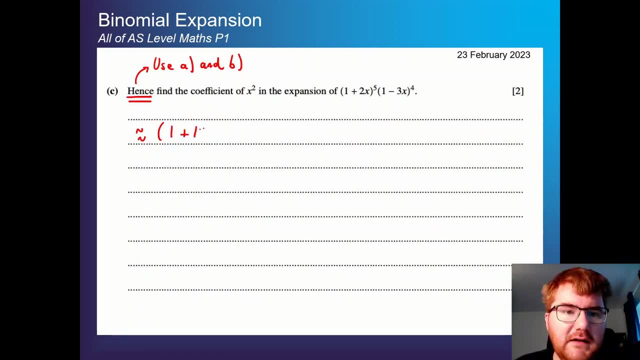 to do is replace those brackets with our estimates that we worked out from part a and b. so I'm going to be using this one right here, and then I've got the first bracket. so 1 plus 10x plus 40x squared, it's dot dot dot, but we don't really mind about that part. then 1 minus 12x plus 54x squared plus. 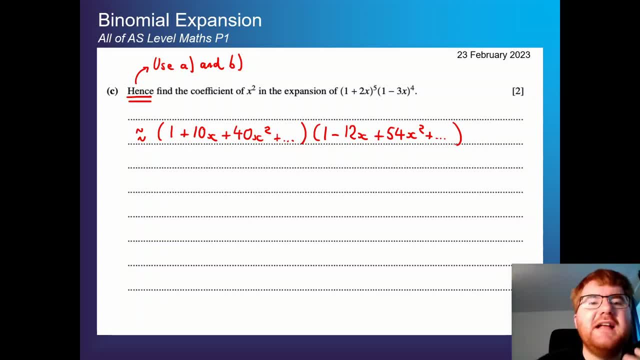 dot, dot, dot. and now we need to consider how can we actually generate the x squared terms. there's only so many ways that we can do this, so we're going to do this by using this one right here, and we're going to do this by using this one right here, and we're going to do this by using this one right here, and 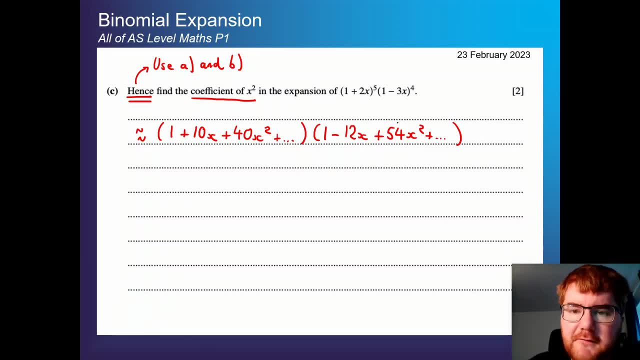 do this, And I'll do this in a different colour. First of all, it's going to be the 54x squared times the constant, so 1.. So those two will generate an x squared term. These two will generate an x squared term for the same reason, because you get x squared times a constant. 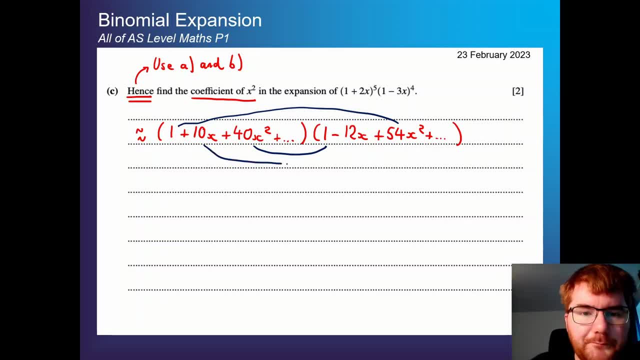 still an x squared term, But don't forget also this term in the middle, because 10x times minus 12x will give you an x squared term as well, And those are the only ways you can generate x squared terms. Notice if we had an x cubed term, that can never generate. 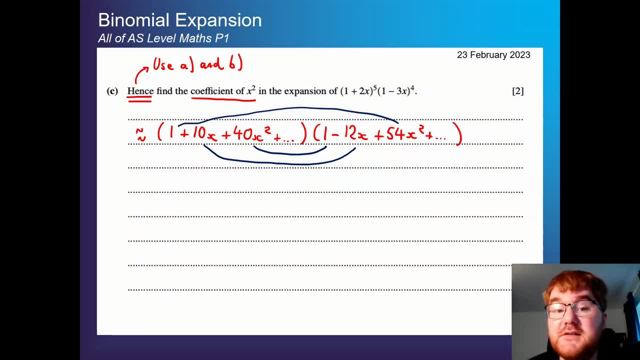 an x squared term, It'll generate one less than its power. So all we need to do is work out these three that I've put here in blue. So we've got 54x squared times 1.. Well, that's just 54x squared. And then we've got 1 in the middle, so 40x squared times 1.. Well, 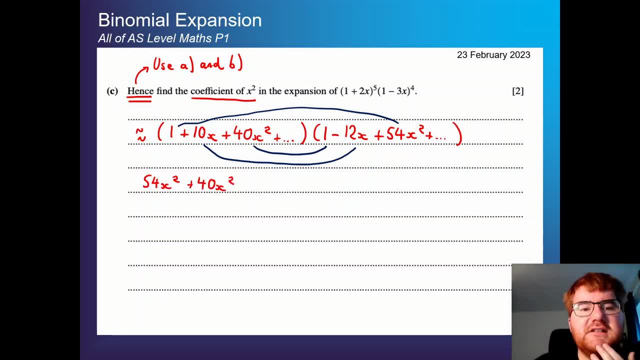 that's just 40x squared, And then we've got 10 times minus 12, so that gives us minus 120x squared, And if we collect up the like terms here, we've got 94 minus 12x squared. 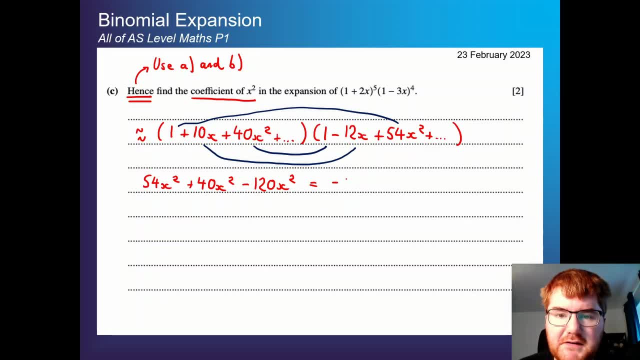 That's 120.. And that's going to be equal to minus 26x squared. So our actual answer here, the coefficient- because that's what it's asking for here- is just equal to this number that we just worked out. So we've got our answer there of minus 26.. Notice this. 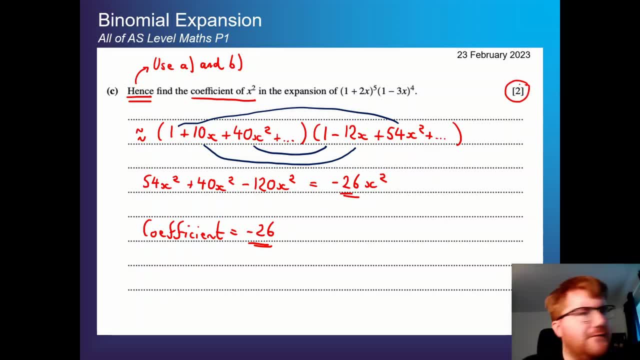 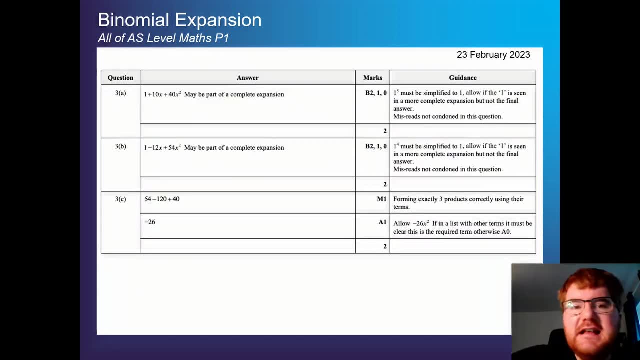 is a two-mark question, so it shouldn't be anything too difficult in order to work out the answer. OK, so you can check you're working there. That's a fairly on the easiest side of the equation and you can do that by looking at the question in this particular video. 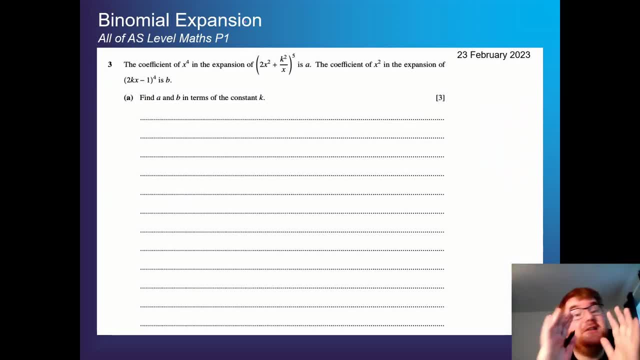 Right on, we go to question three. It looks scary. when you see this, You go: oh God, what do I need to do? But don't worry, Just take it one step at a time and you'll be absolutely fine. So the coefficient of x to the power of 4, important. underline this. 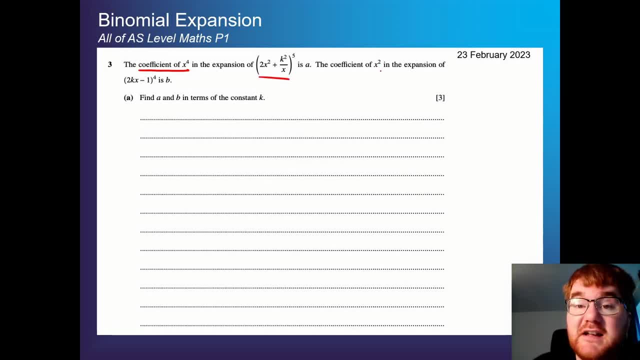 of this bracket is a and the coefficient of x squared in the expansion of that bracket is equal to b. OK, So we've got our answer here. So we've got our answer here, And we need to work out a and b in terms of k. OK, because we have k in both. So if we take the nth term formula, 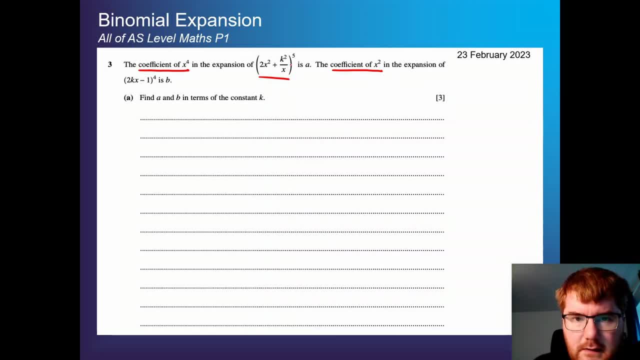 we want x to the power of 4.. This is going to be a bit tricky because we've got an x squared term here and we've got an x term here. So what I'm going to do- just to show you the process, because we're going to be using this idea a bit later on- is actually: 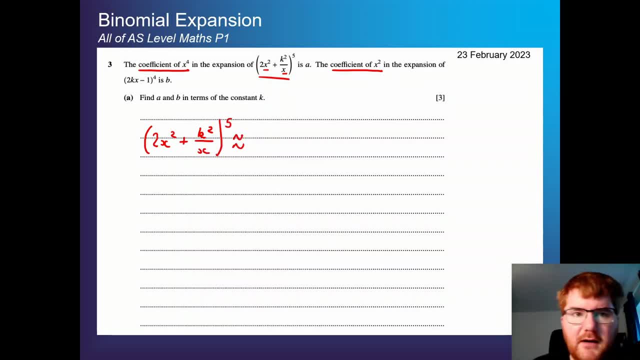 expand this normally, without really considering that part for the moment, And then we're going to come back to it. So if we approach this in the same way, first of all we just get the first term, which is our 2x squared to the power of 5.. Then we're going to have 5. 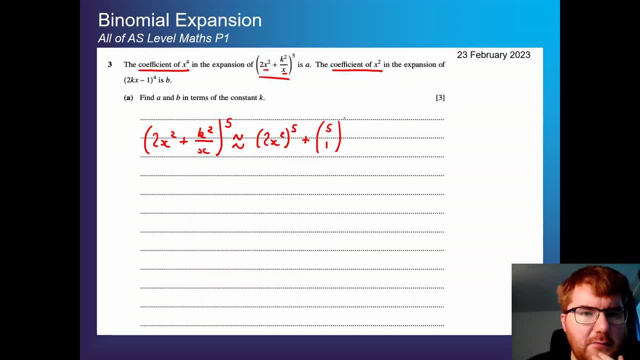 choose 1.. And then we've got 1 less on that index, So 2x squared to the power of 4.. And of course we'll also have 1,, 3,, 4,, 5,, 6,, 7,, 8,, 9, and 10.. 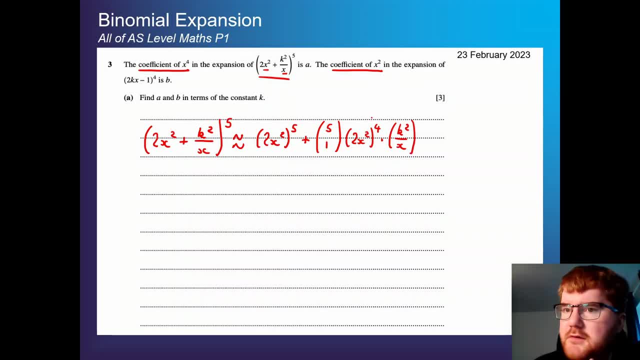 So we've got this term here and we're going to try and get rid of that first term, And we're going to have our x squared to the power of 5, and then we're going to have our two next. So we're just going to keep adding and subtracting these two terms, or we can do. 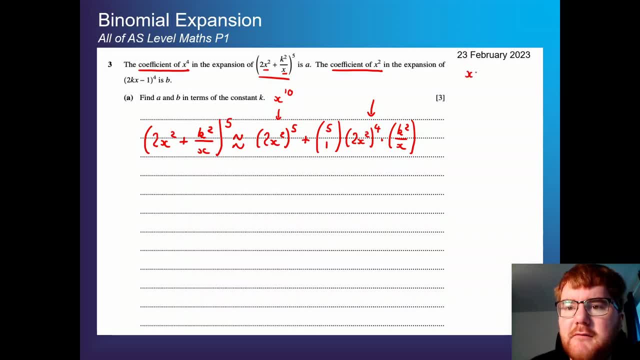 it in other ways, And this is going to give us our first term, which is our 2x squared to the power of 4.. OK, and we don't really need to add to this. We don't have to add to this. We don't need. 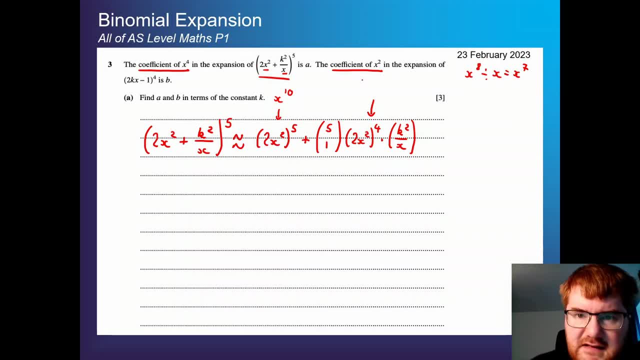 divided by x is equal to x to the power of 7.. So this gives me an x to the power of 7 term And we want x to the power of 4.. So if we do the next one here, so we go 5 choose. 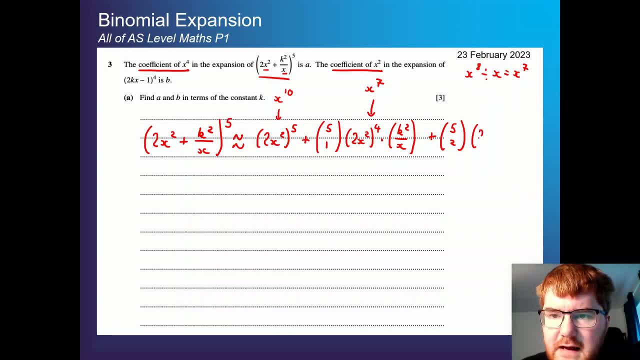 2, 2x squared to the power of 3, k squared over x squared. If we consider this term now, we have x squared to the power of 3, that's x to the power of 6.. This one here is then. 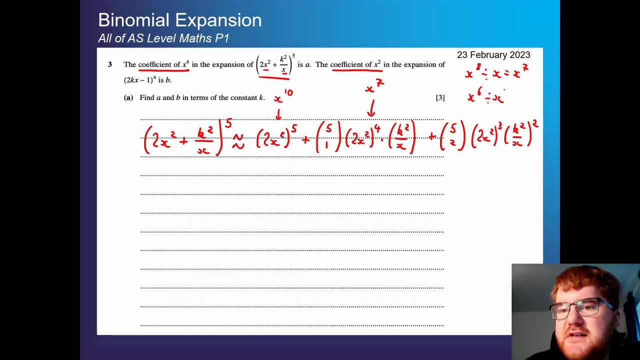 going to be over x squared, And if we do x to the power of 6 divided by x squared, we get x to the power of 4.. So it's this term here that I'm going to highlight that, once we expand this out- and you probably need to see this a couple of times to believe it- 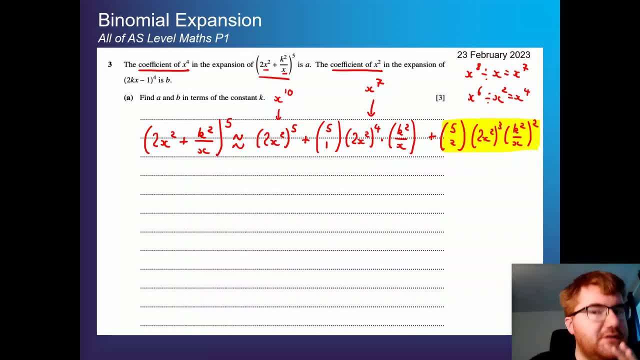 is going to give us the x to the power of 4 term. Now again, we've done that by a sort of trial and error method. As you go into subsequent questions you'll see you can spot these a bit quicker. But just to give you an idea, just expand it out. 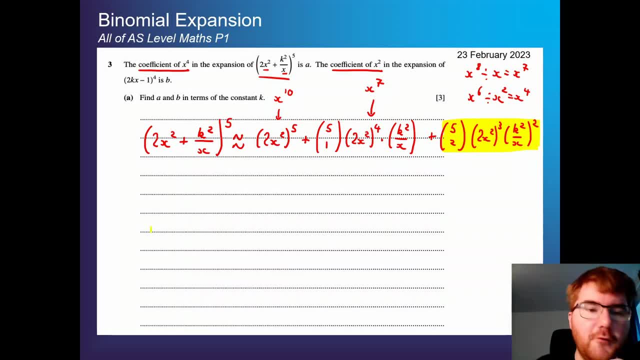 because only up to 5, and then see which term actually gives you x to the power of 4.. Now we need to actually work this out. So if we work out 5, choose 2, 2x squared, all cubed. 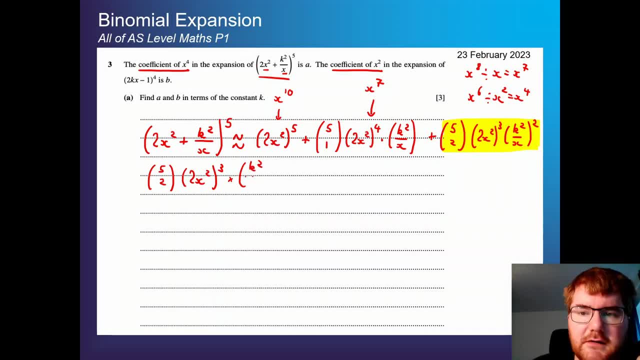 and then times k squared over x, all squared, Now 5, choose 2, we already worked out that was equal to 10.. So we can put that in here. So we can put that in here. So we can put that in here. 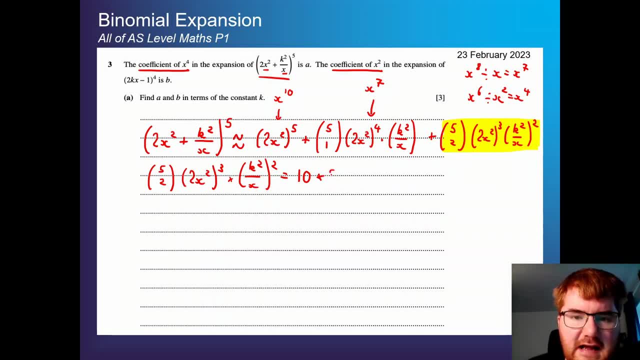 So 10, 2 cubed is equal to 8.. k squared all to the power of 2 is equal to the power of 4.. And we already worked out the x squared, what happened to the x terms, And that will be then. 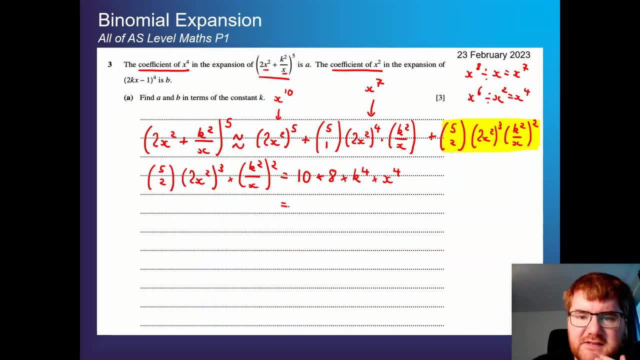 x to the power of 4, which is what we wanted. If we simplify this, then we're just going to get ourselves 80k to the power of 4, x to the power of 4.. And we're told in the question this: coefficient here, 80k to the power of 4, is equal to 80k to the power of 4.. And we're told in the question: this coefficient here, 80k to the power of 4, is equal to 80k to the power of 4.. 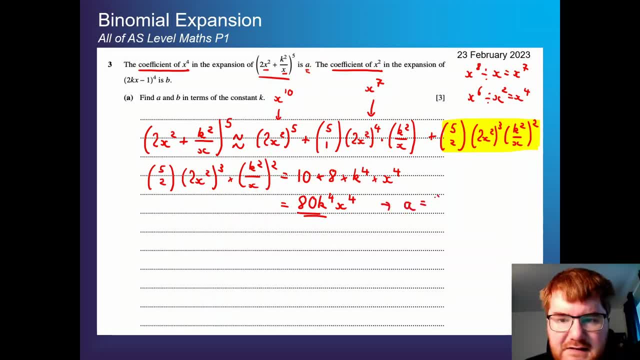 And we're told in the question, this coefficient- here, 80k to the power of 4, is equal to 80k to the power of 4.. So let's just write it down very clearly for the examiner: a is equal to 80k to The power of four. 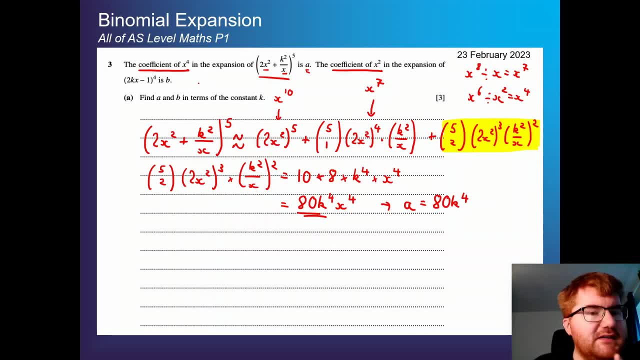 Now B. we can do in a very, very similar way. we can speed this process up slightly, And let me just show you how we can do that. So this is the expansion that we want to focus on. We want the x squared term. Well, the very first term will be x to the power of 4.. 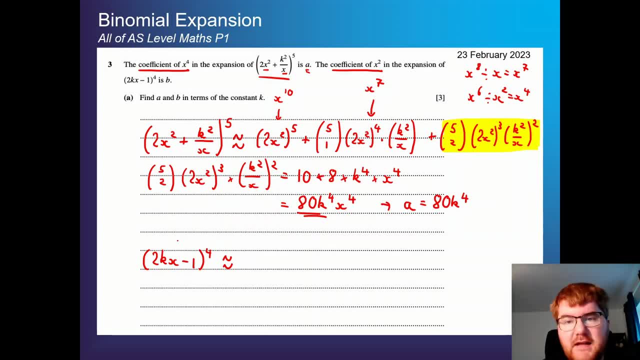 The next term will be x to the power of three, because you reduce one down. The next term will be x to the power of 3, because you reduce one down. So the third term will be x to the power of 2.. So we can kind of cheat here and go straight to this term 4, choose 2.. 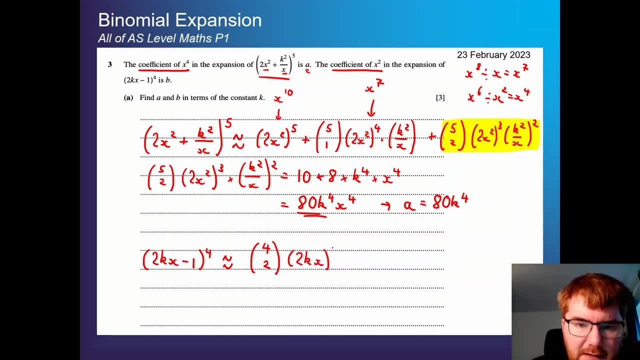 We go 2kx to the power of 2, because 4 minus 2 is 2., And that's what we wanted- And then multiplied by minus 1 to the power of 2.. So this is the quick way of doing the process, rather than that longer way which I showed you in the previous part. 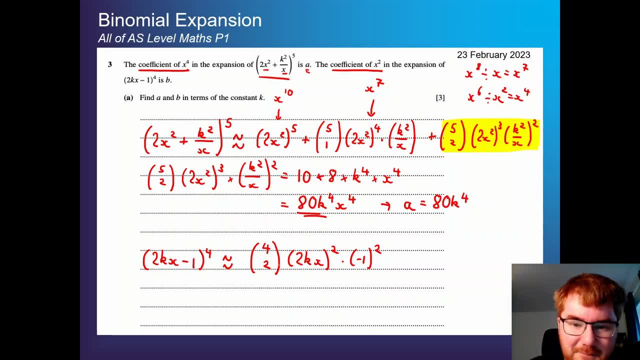 Now 4 choose 2, I've still got on my calculator from the previous question. So that's equal to 6.. So you've got 6 times well, 2k. all squared, that's going to be 4k squared. 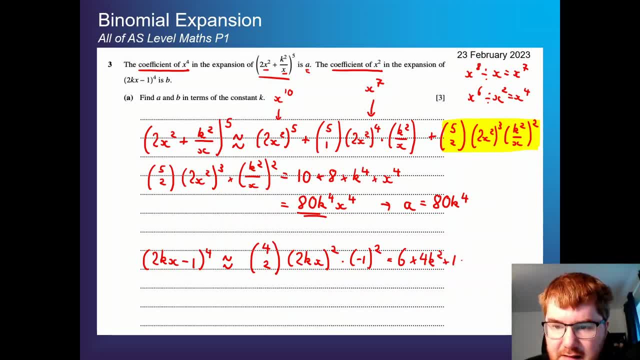 Minus 1 squared is just 1, so that's nice, And then we get the x squared that we wanted. So that's going to simplify down then to 24k squared, x squared, And the question. they say that this coefficient is equal to b. 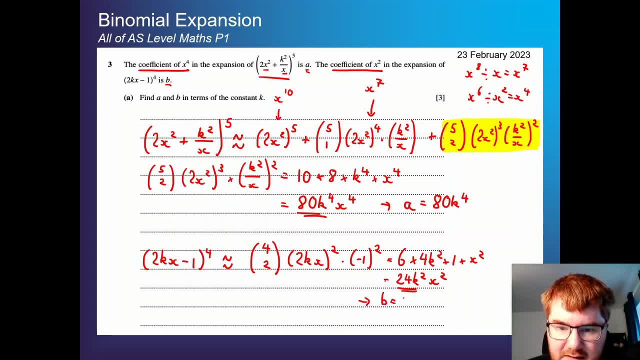 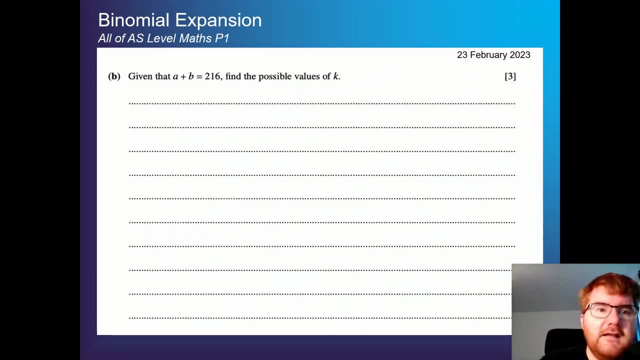 Therefore, let's make it nice and clear for the examiner: b is equal to 24k, b is equal to 24k squared, And that gives us our three marks here. Now, very typical, there's always a follow-up question to this general expansion. 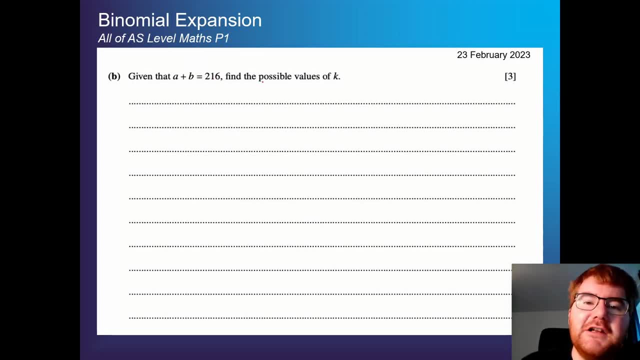 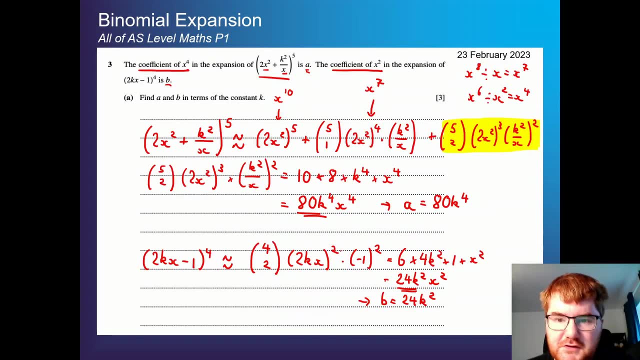 Given that a plus b is equal to 216, find the possible values. Again, I see values- I'm thinking quadratics and cubics- to solve this. Now we know what a and b are, because we just worked this out. 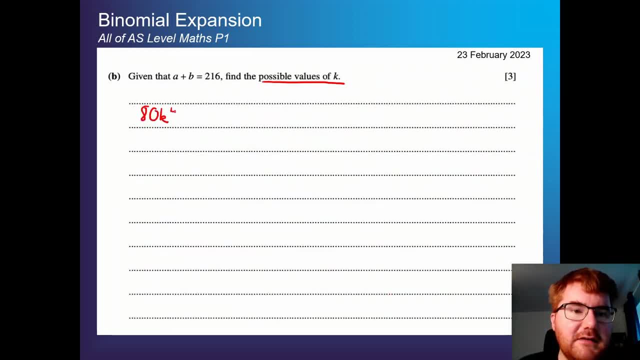 So a is 80k to the power of 4.. b is 24k k squared and that's equal to 216.. Right, so again solving this. again, we want to make the right-hand side zero, So we're just going to minus 216 from both sides. 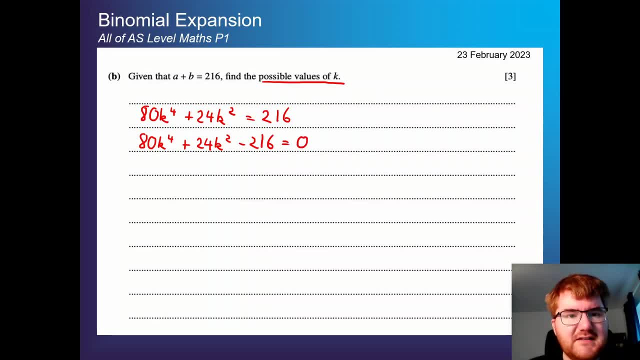 At the moment, this looks like a fairly complicated quadratic to deal with or quartic to deal with. The first thing that comes to mind is trying to simplify this down, And we can do this by dividing by 8 on both sides. And we can do this by dividing by 8 on both sides. 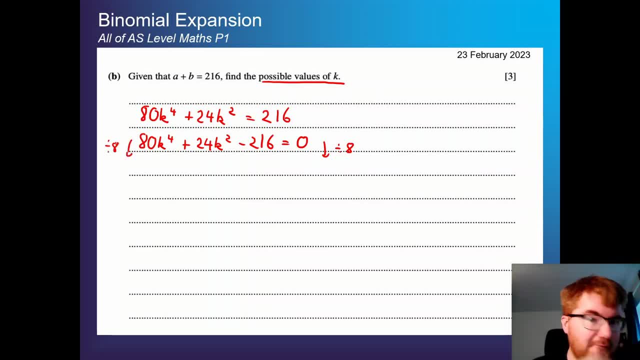 If we can find any process that makes it a little bit easier for us, we should try and take it. So we divide everything by 8. here We get 10k to the power of 4 plus 3k. squared, And dividing that was 27 is equal to 0.. 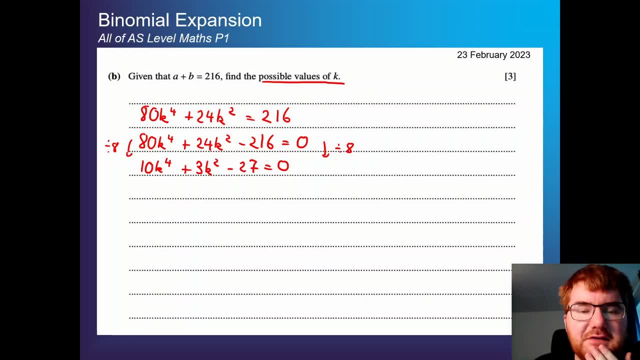 Now. I showed you by substitution last time how to do this. I'll do it by substitution again here. So we're going to do: let u equal k squared. Remember that trick that we did in the previous question: Start seeing patterns. We're going to start seeing patterns with this kind of video. 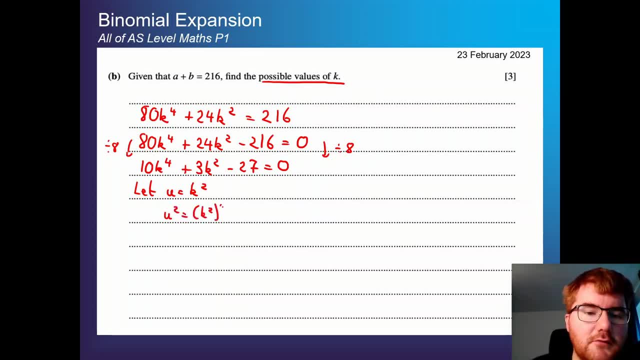 Therefore, u squared will be equal to k squared, all squared, which is equal to k to the power of 4.. Pop this in. We then get a quadratic. we can work with: 10u squared plus 3u minus 27 is equal to 0.. 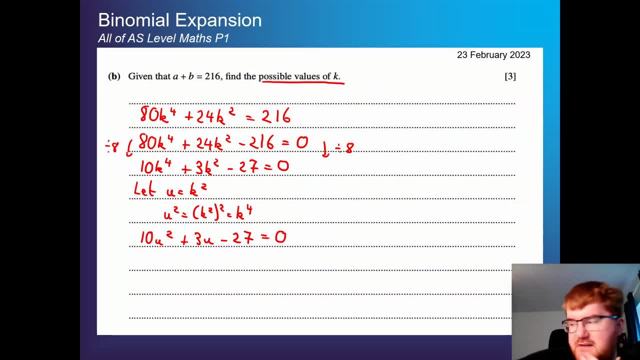 Again, at this point there are a few choices we can actually put inside our brackets. So again, we look to try and factorize if we can. Let's have a think about this. So 27, it's factored. 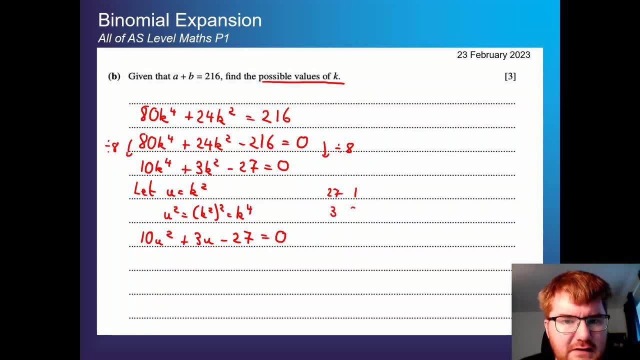 We've got 27 and 1.. We've got 3 and 9.. I don't think anything else goes there. So generally my strategy here is: just try something else. So we're going to do 5u and 2u. 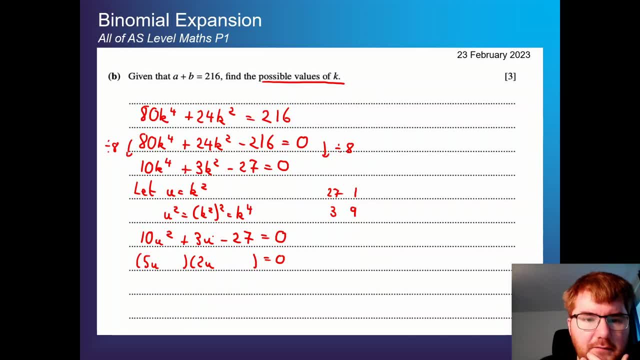 See if we can make 3 from 9 and 3.. 15, 18.. Yes, we can. So if we put and we want positive, So that's 9 there And minus 3.. Again, what I'm doing in my head is essentially I'm checking these cross terms. 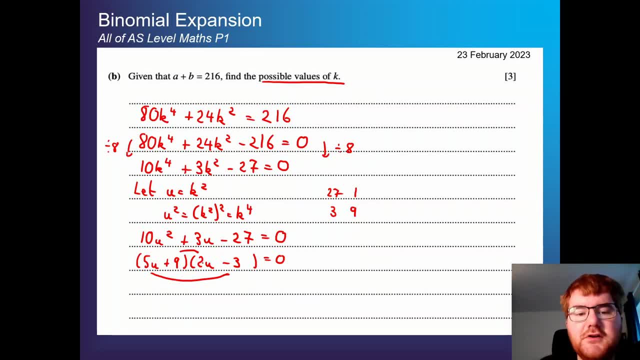 5u times minus 3 is minus 15u. 9 times 2u is equal to 18u Minus 15u. plus 18u is plus 3u. Yes, we've got what we wanted. If you're wondering why I chose 5u- 2u straight away, from experience, they generally do choose numbers quite close to each other. 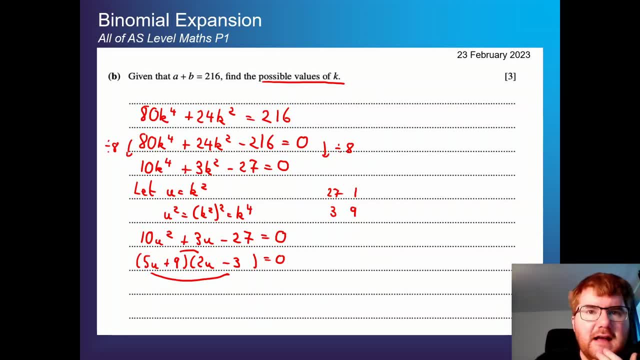 10u and u. that comes up less often than you think. So again, this just comes from experience. The more questions you do on this, The easier to get. Now, at this point, we're going to need to solve this. 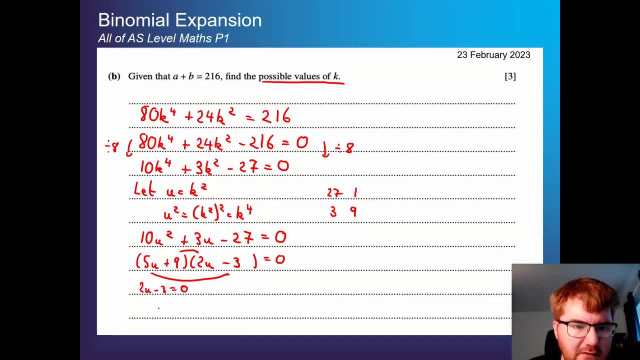 So therefore, 2u minus 3 is equal to 0.. So u is equal to 3 over 2.. Or 5u plus 9 is 0. Therefore u is equal to minus 9 over 5.. 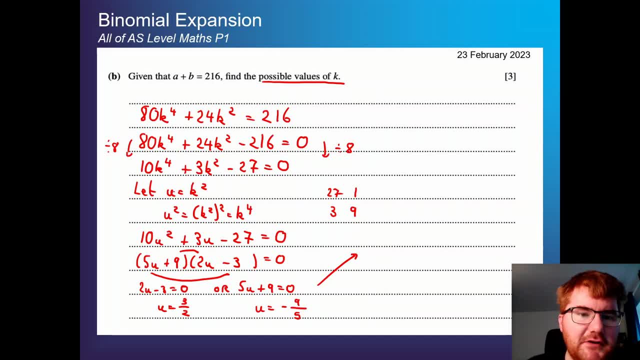 However, remember we need to back substitute here, So we're now replacing the u back with k squared, So we get: k squared is equal to 3 over 2.. Or k squared is equal to minus 9 over 5.. 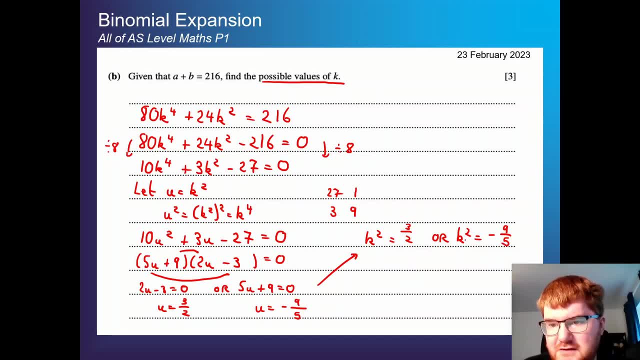 Ah, So if we try and square root this second one here, then that's not going to work. We get complex numbers Again, so this one doesn't work. So our only answer here is going to be plus minus square root of 3 over 2.. 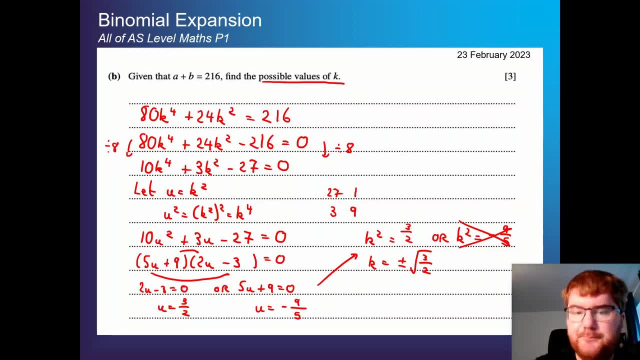 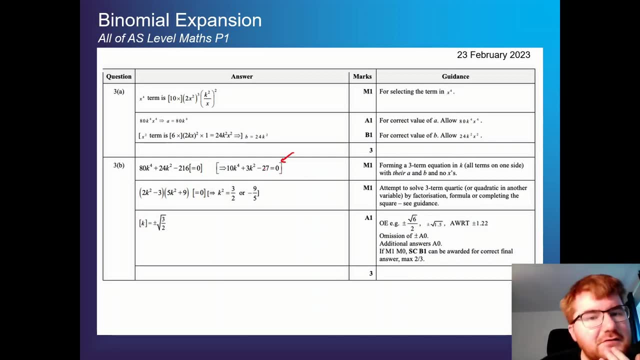 So this one in particular has only got two answers, So you can check all the working that I've done there. I did take this approach here of simplifying. I did take this approach here of simplifying down and factorizing. 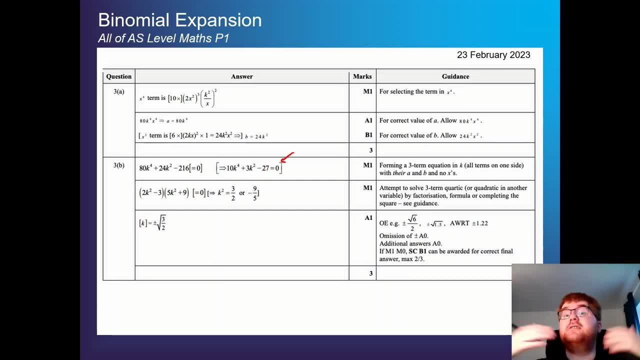 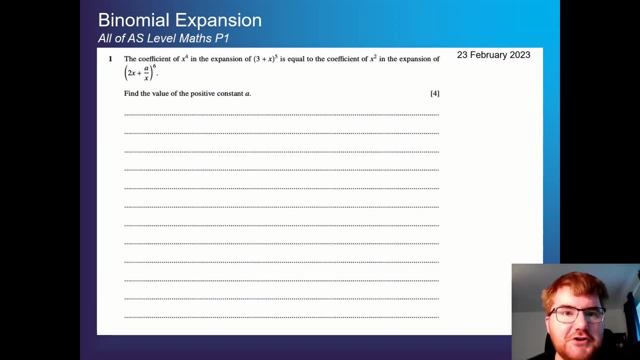 I think that was an easier way to go than try and head straight into the quadratic formula, which is not always the most fun thing to do in the world. Okay, And on to the next question here. So the coefficient of x to the power of 4 in this expansion. 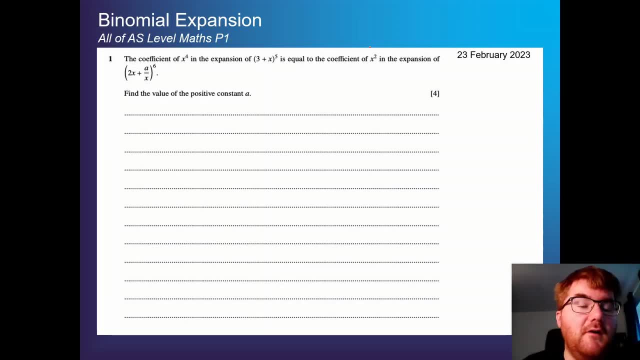 ah is equal to the coefficient of x squared in the expansion of the other bracket, and find a Very, very typical This whole equating two coefficients. We haven't seen this yet in this video, but it does come up quite often. 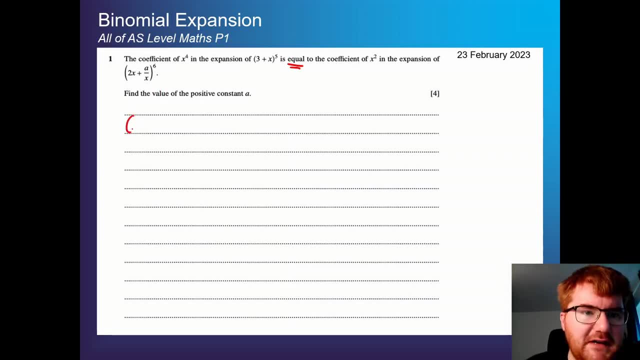 So let's try and speed up the process. going through this Now you've seen a lot of the theory, So 3 plus x to the power of 5 here And we want to find the x to the power of 4 term. 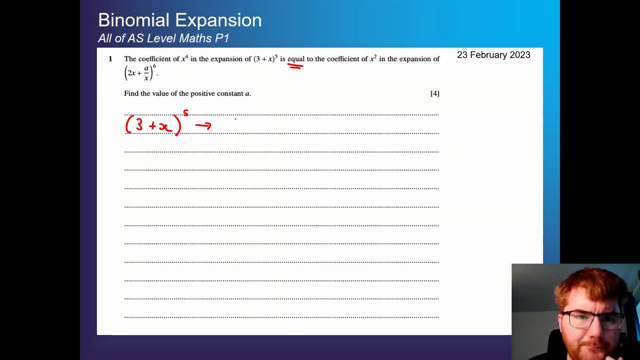 Right. So in order to find the x to the power of 4 term, we want this to then be 5, choose 4. Because that's going to make this term x to the power of 4.. If you go right back to the formula, 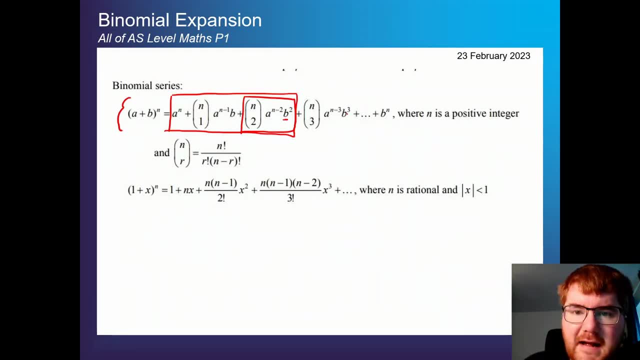 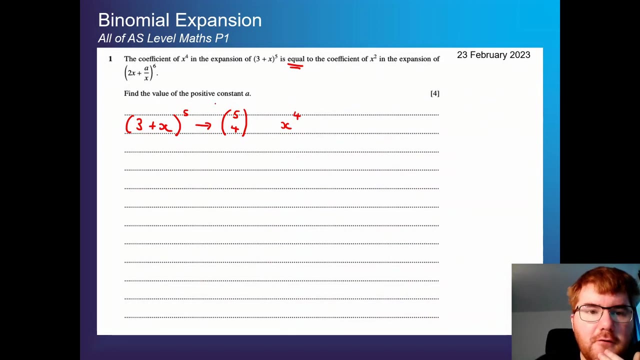 what I'm doing here is I'm matching this here with this number here. So that's how I'm matching up the binomial coefficient with the actual power. So go right forward through. There we are. So we've got 5. choose 4, x to the power of 4.. 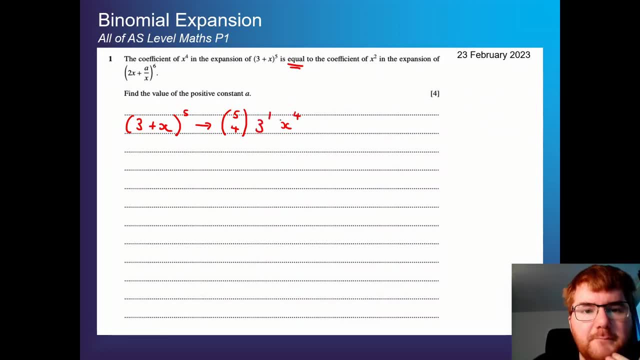 And because this is 4, this one has to have a power of 1.. 1 plus 4 is equal to 5.. So if we work this out, let's work out 5, choose 4 in the calculator, So 5.. 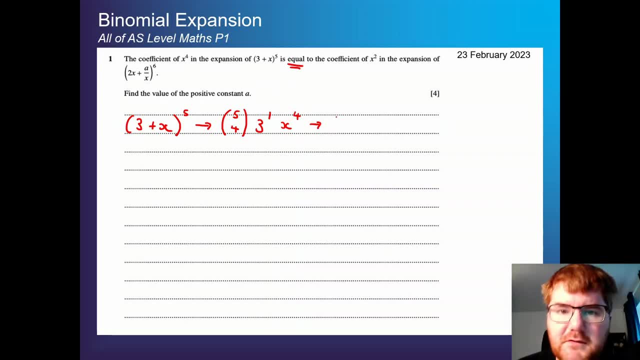 Choose 4.. That's equal to 5.. So we get 5 times, 3 times x to the power of 4. And that gives us 15 x to the power of 4.. Okay, We'll come back to that in a moment. 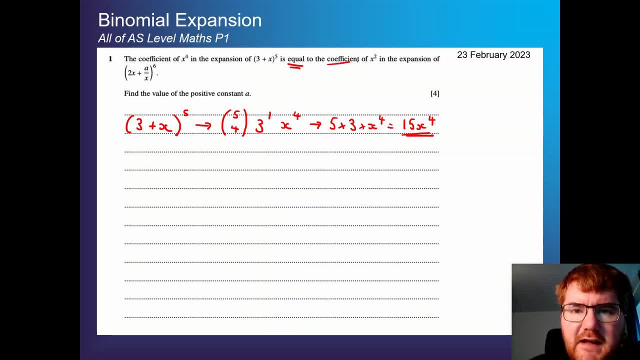 And now we need to do this one here. So now we've got the coefficient of x squared in this expansion. Okay, Now this is a bit more complicated Because we've got an x term here and an x term here as well. 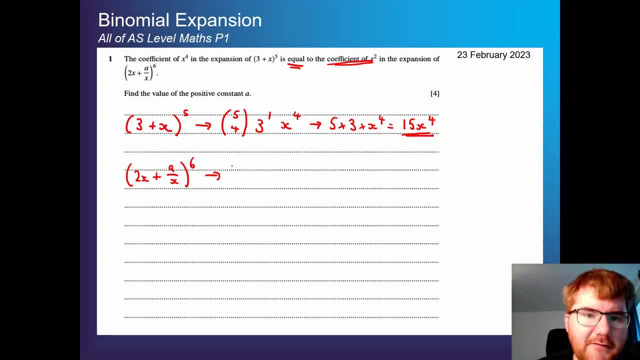 So let me just try one out. So if I was to do, for example, 6 choose 2.. I'm not saying it's the right answer, but I'm going to do 6 choose 2.. Then that means then this one here has to be a over x all squared. 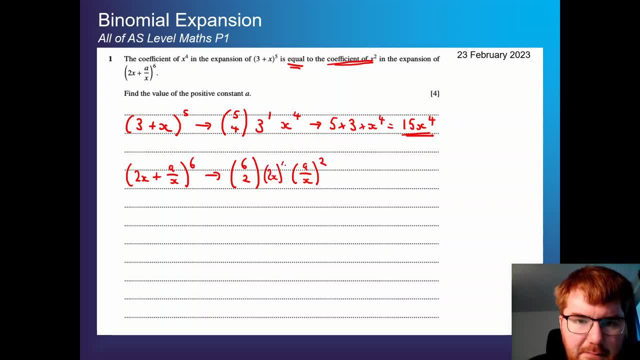 And that means that this has to be to the power of 4.. And then we get x to the power of 4. divided by x to the power of 2 gives us x to the power of 2.. Great, That's exactly what we wanted. 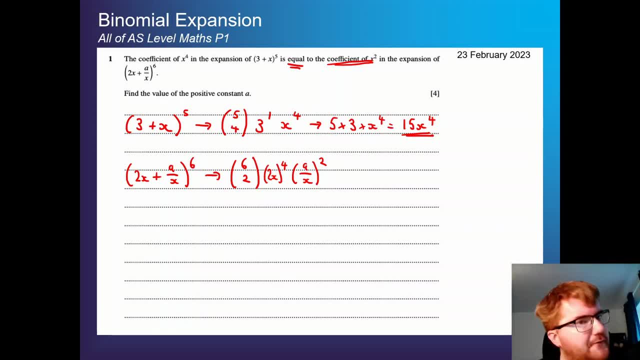 Again, this is the kind of process you can do If you didn't get that straight away, and try 6 choose 4,, for example. you'll get the wrong answer, But then you need to learn from it. Now, if we work this out, then 6 choose 2.. 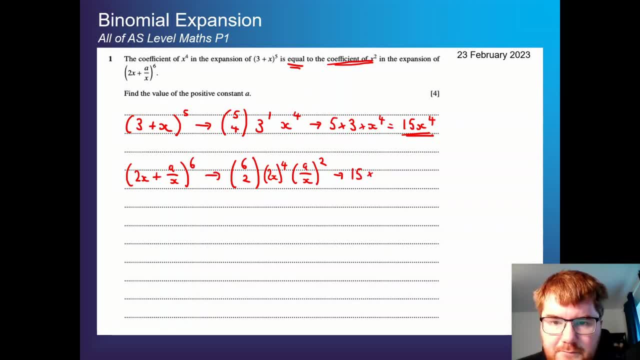 That's equal to 15.. So we get 15.. 2 to the power of 4 is equal to 16.. a squared is just a squared, So that's fine. We can leave that as it is. And then we check the powers here already. 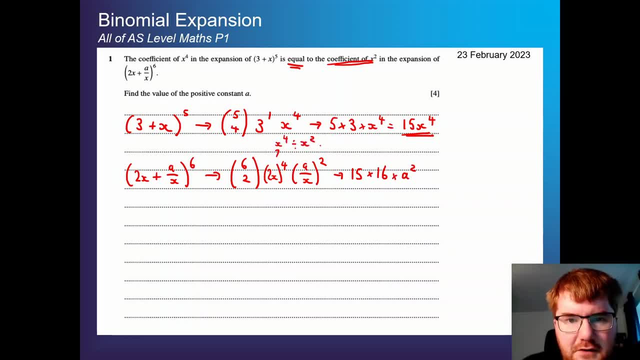 So x to the power of 4.. This is going to be divided by x to the power of 2.. And that gives you x to the power of 2, which we wanted. So this gives you this here, And then 15 times 16 is 240. 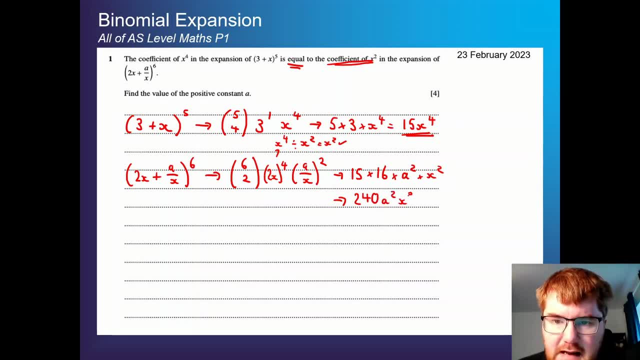 So we get 240 a squared x squared, And the question says that the coefficients- So remember the coefficients here, That's the 15. And the 240 a squared, are equal to each other. Therefore, we can just say here that 240 a squared is equal to 15.. 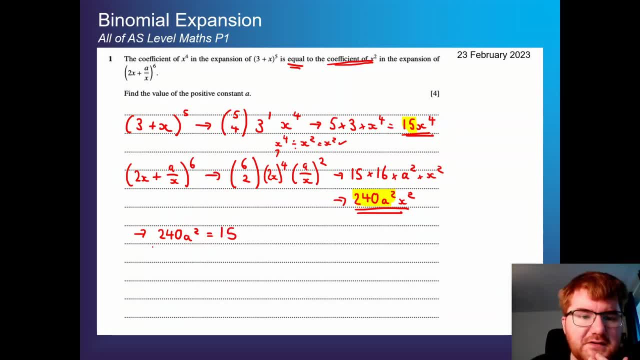 And this is now just a straightforward quadratic to solve here. So we're going to get the a on its own- Excuse me- By dividing by 240 on both sides. This cancels giving us a squared, Now 15 divided by 240.. 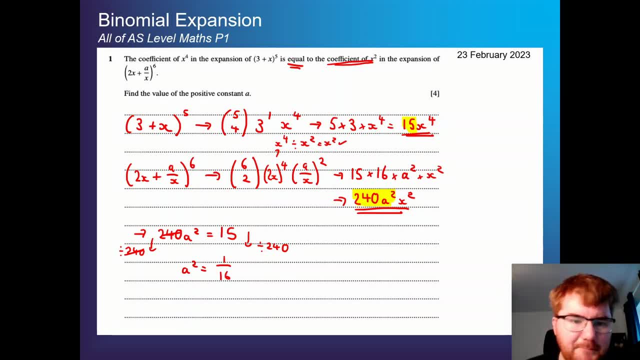 240.. Aha, that's equal to 1 over 16.. That's a very good sign. And now we're going to square root both sides. It's the opposite of squaring: This cancels, We get a, And then we get plus, minus the square root of 1 over 16.. 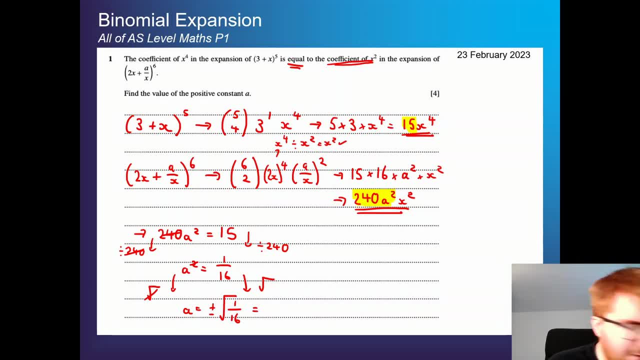 And if we do that- you can just do that on your calculator- You're going to get yourself plus minus 1 over 4.. However, you need to read the question carefully. We want the value of the positive constant a, So therefore our final answer will just be equal to a quarter. 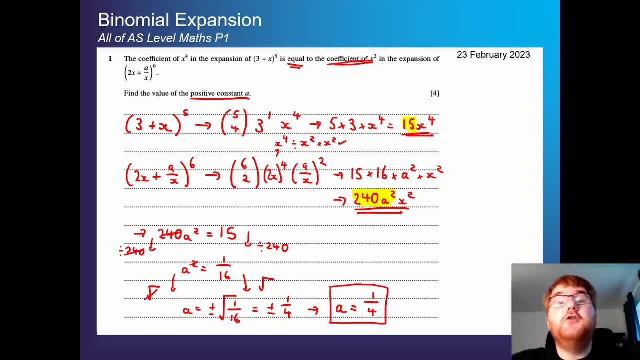 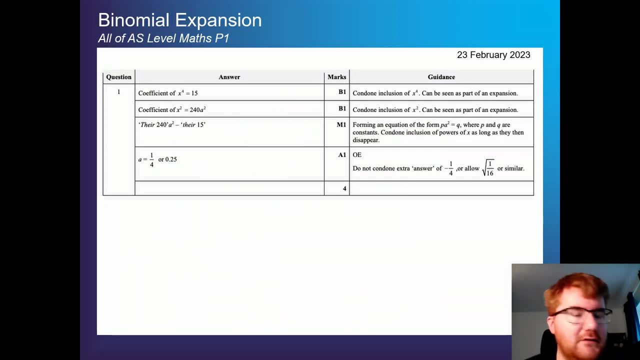 Again, you need to make sure you're reading the question really carefully So you're not missing out on every single mark on this kind of question. Right, You can check your answers there and look through everything that I've just done. And on to the next question. 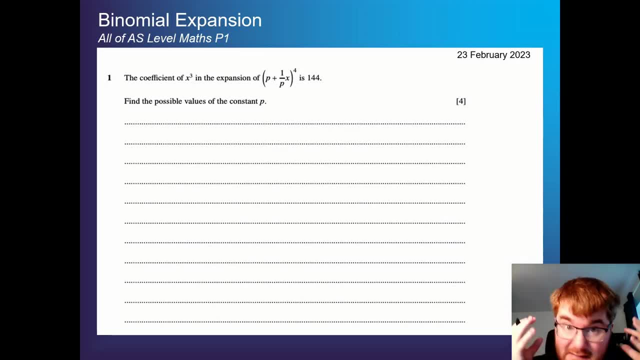 Again, this is the way to really get good a particular topic: Just practicing lots of questions, Listening to my voice as I go through these questions And trying them yourselves as we go through. So the coefficient of x cubed in the expansion of p plus 1 over p x to the power of 4 is 144.. 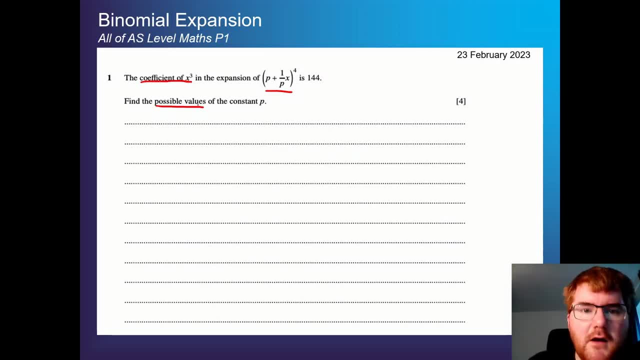 Find the possible values again. Again, I'm always looking for that Of the constant p Right, So let's open up p plus 1 over p x to the power of 4.. And we want the x cubed term. 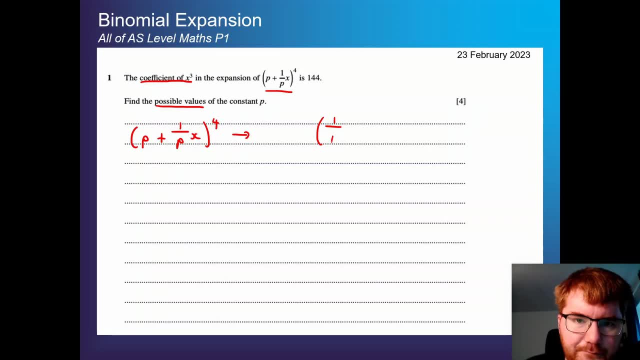 Therefore, I'm sort of working backwards here. So I want this To be cubed. If that's cubed, then we want to use 4 choose 3.. And if we want 4 choose 3, then this needs to be p to the power of 1.. 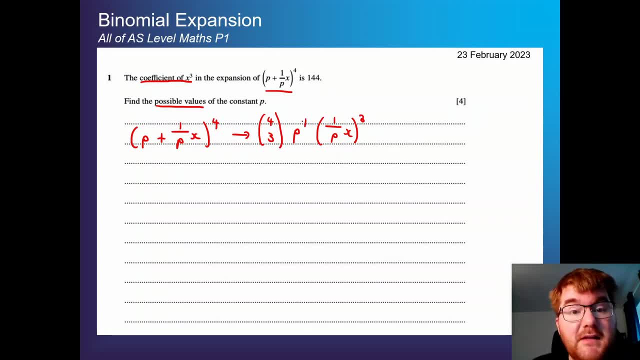 So it's a way of working backwards. I know I want the x cubed term, Then I know what the binomial coefficient is And I know what this term here is as well. Okay, So 4, choose 3.. 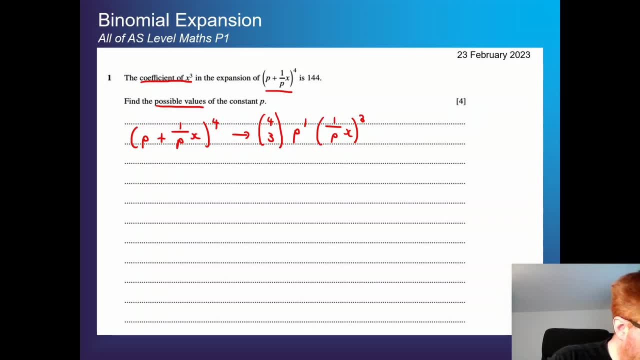 We can work that out very quickly Again using our calculator. It gives us 4.. So we get 4 times p times 1 over p all cubed. That's just going to be 1 over p cubed. 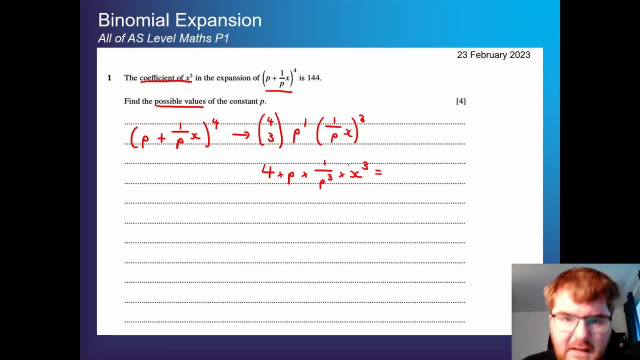 Excuse me, Times x cubed. If we simplify this down, We're going to get some cancellation here. So we get 4 over p squared x cubed If we simplify this down And this coefficient that we worked out. 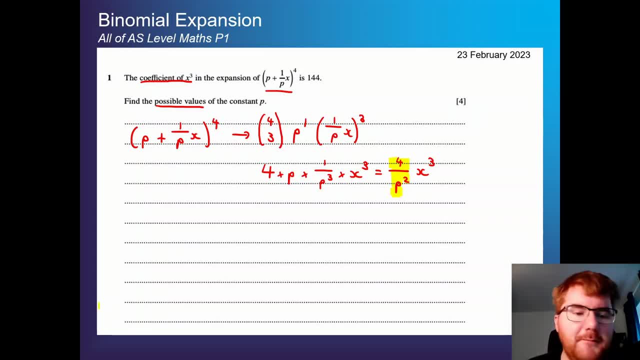 Remember, p is just a constant here, It's just a numerical value That's going to be equal to 144 in the question. Therefore, we can just say that 4 over p squared Is equal to 144.. And this is now just an equation to solve here. 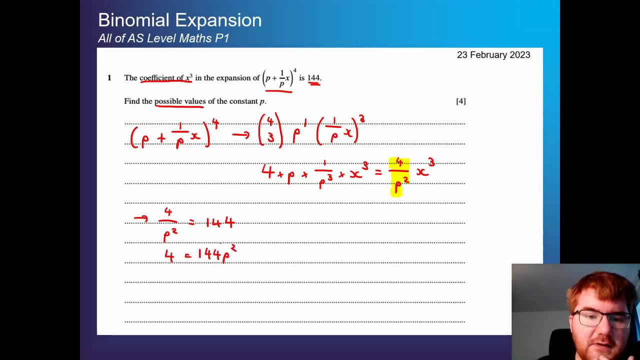 So we get: 4 is equal to 144.. p squared: p squared is equal to 4.. Divided by 4, divided by 144.. So if we pop that into the calculator, Yep, we get something very nice. 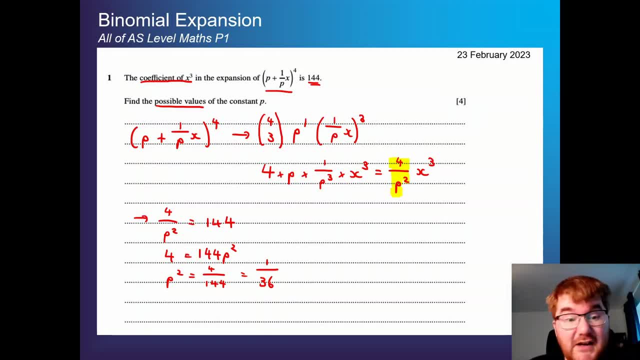 Again, if I'm getting 1 over 36.. I know it's going to square root really nice, So I'm probably on the right lines. And therefore p, If we square root both sides, It's going to be the square root. 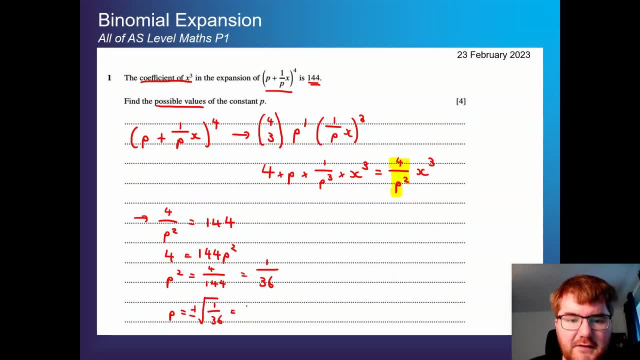 Of 1 over 36.. And that's going to give us- You can check on your calculator here- Plus minus 1 over 6.. Notice, in this question, Compared to the previous one, They just want the constant p, So they haven't said the positive or the negative. 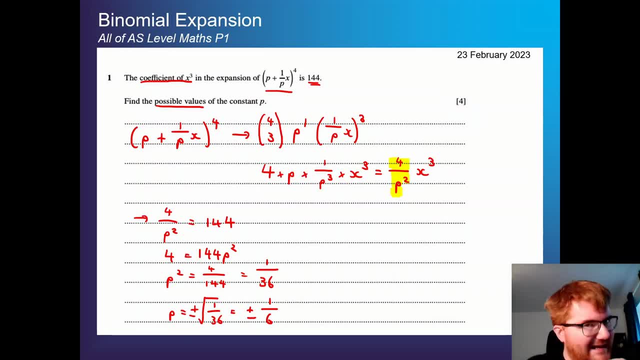 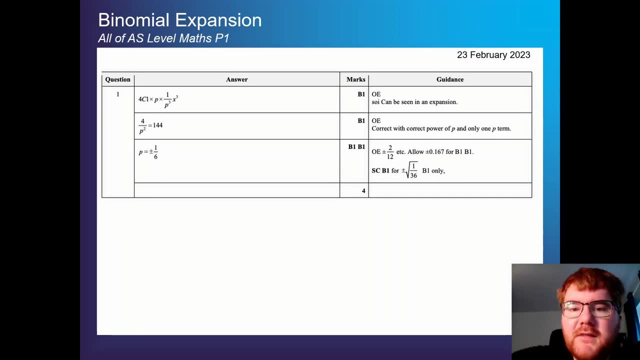 So you do need to give both plus and minus When it doesn't say anything specifically. So that was a nice question. Again, the question 1.. Typical Start a question for a paper 1. And you can check all the working there as well. 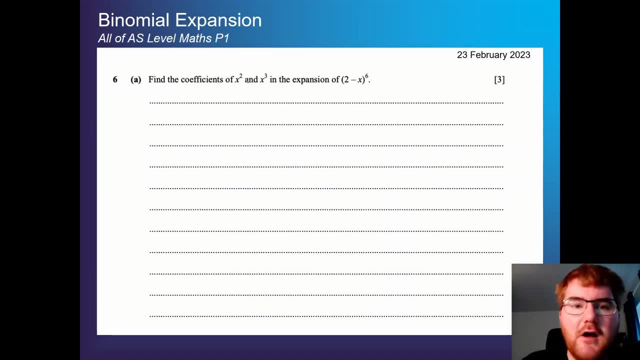 And on to our next question. So we're going to find the coefficients Of x squared and x cubed In the following expansion, Right? so We've got 2 minus x To the power of 6. Again, we can. 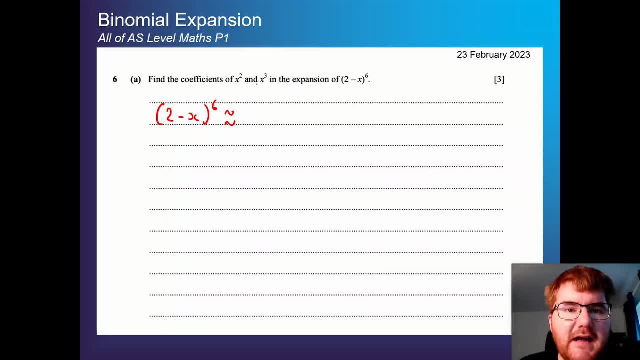 Go specifically into these ones. So we're looking for x squared. Then we know that term there Needs to be To be squared. Therefore, This needs to be 6, choose 2.. This needs to match And that gives you 2 to the power of 4.. 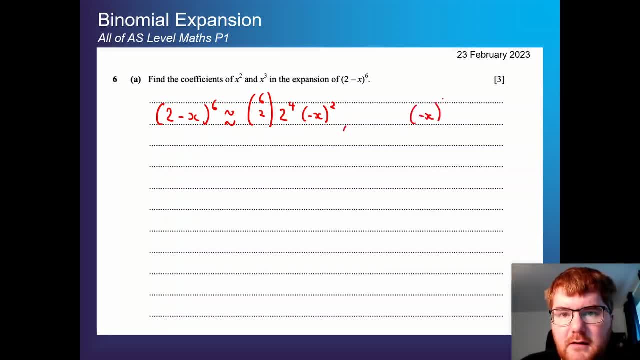 And then, Likewise, We've got minus x to the power of 3. That matches with 6. choose 3.. That gives you 2 to the power of 3.. 3 plus 3 is 6.. Okay, So if we work this out then, 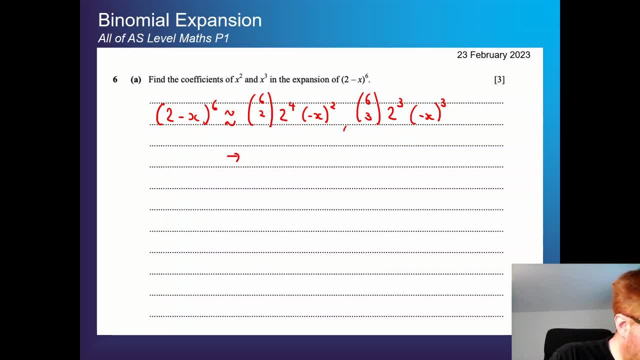 6 choose 2.. I think I've already worked out 6 choose 2. In this video already. So we get 15 times 2 to the power of 4. That's equal to 16.. Minus x. 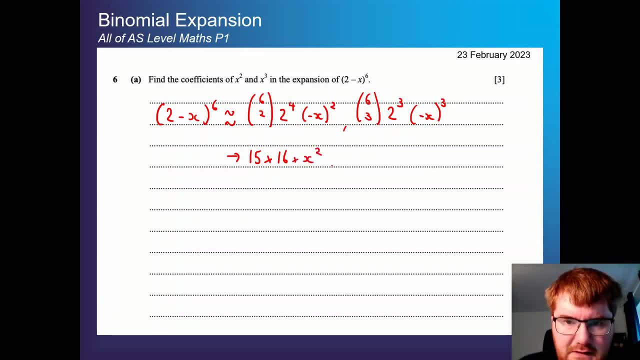 All squared, This is going to be x squared. 6 choose 3.. So 6 choose 3 is 20.. So we get 20 times 8.. Times minus x cubed- Notice a cubic Still going to be a minus there. 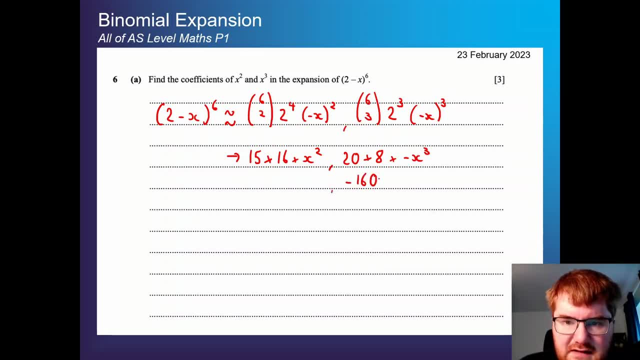 And that gives us then Minus 160 x cubed For that one, And then 16 times 15. Which I think we did that calculation before. Yeah, It gives us 240 x squared. So just going to highlight our coefficients here. 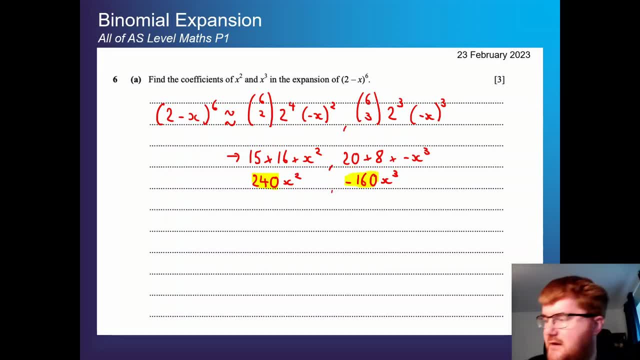 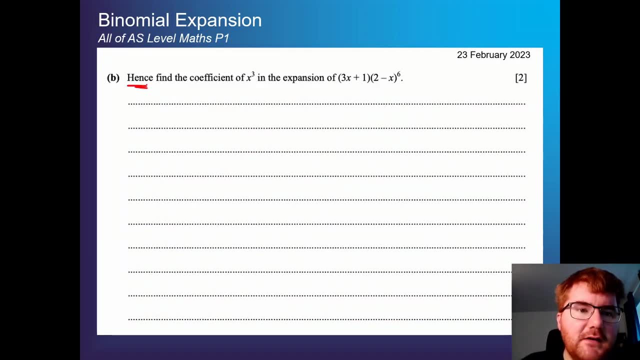 So 240 there And then minus 160 there, Perfect, And hence Again that word, hence again. So using part a, So using part a. That's really important. That's really important Find the x cubed term in this expansion. 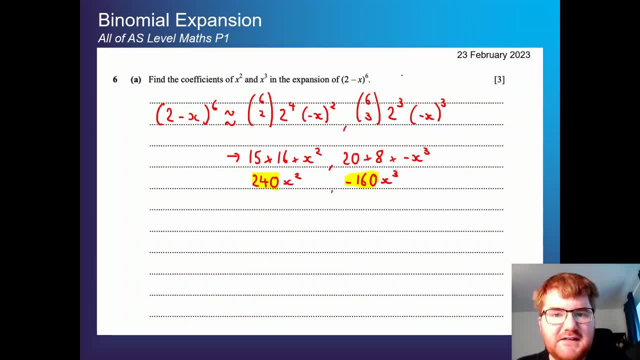 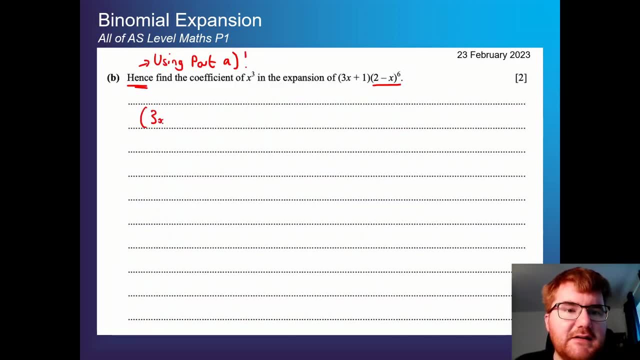 Now notice, we've just been working with this one here. So 2 minus x to the power of 6.. So I'm just going to replace it with the two terms that we have. So we get 3x plus 1.. 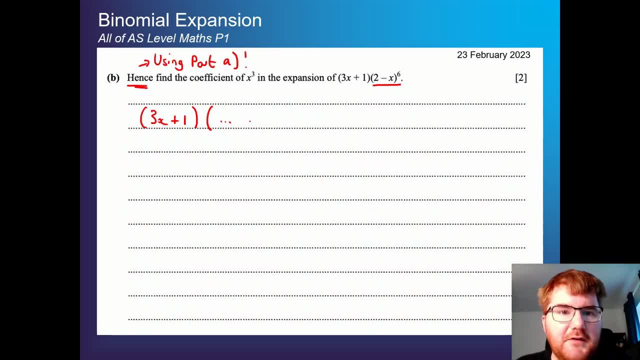 And we have some other terms. That's why I'm putting a dot dot dot, But then we've got the 240 x squared To use. hence, you have to be using what you've already worked with And we want to work out the x cubed term. 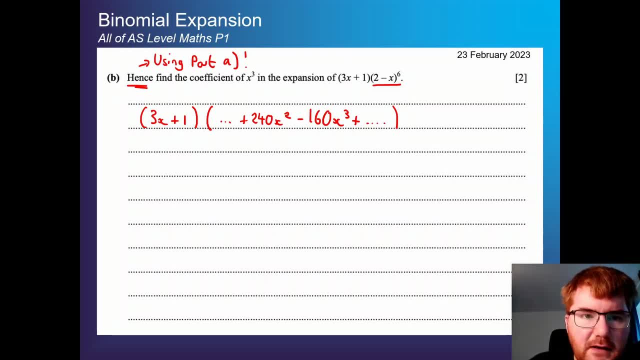 So the only way we can generate an x cubed term is by multiplying this one by this one And this one by this one. So if we do that, we're going to get 240 times 3.. That's going to give us an x cubed term. 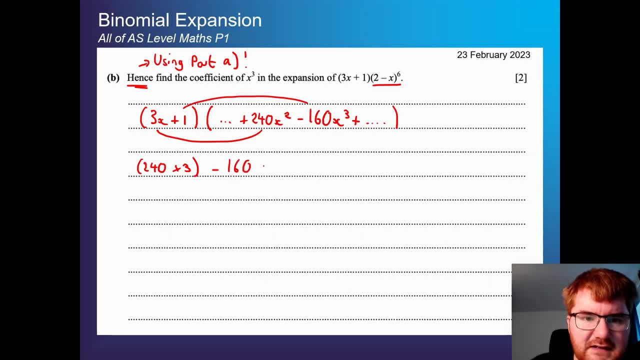 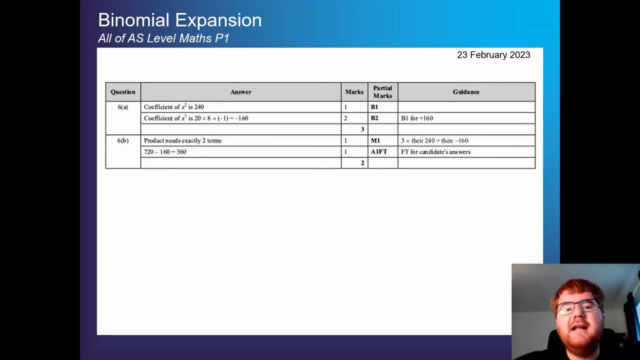 And then minus 160. And if we work this out, I think we get 720.. 720. Right, 160. That again gives us 560 for the two marks Again. so another fairly straightforward question. But the key thing to realise in that particular question there is that you need to be using part A to help you with part B. 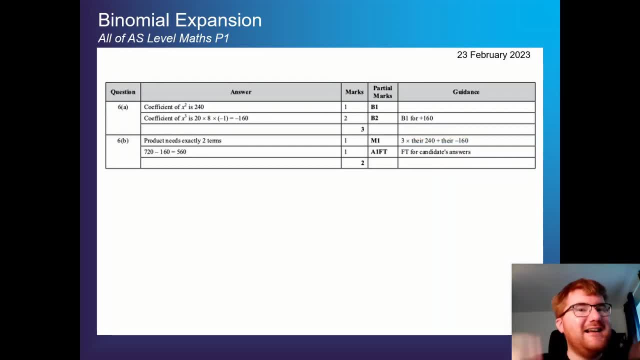 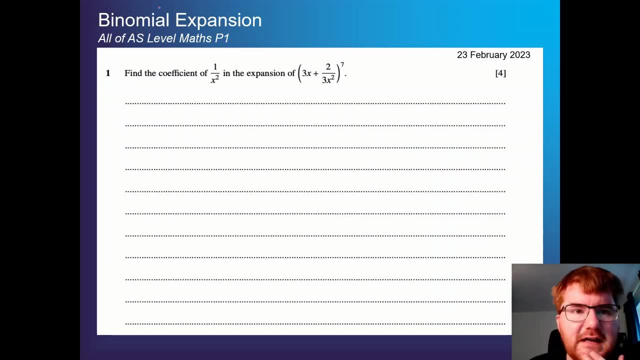 You don't want to be writing out all the expansion and then realising, ah, I could just have used part A, So please do save yourself time in the exam. Right, and our very last question here. So we're going to find the code. 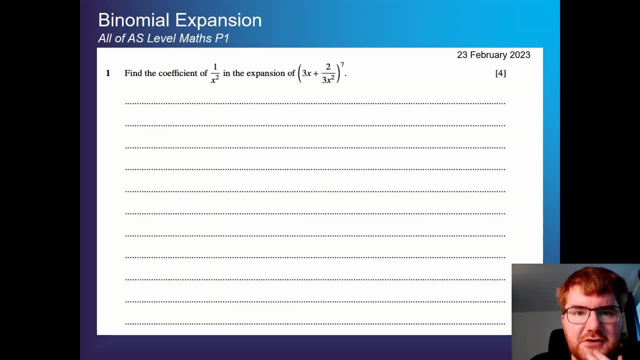 What's the coefficient of 1 over x squared in the expansion of this Right? so Have you got any hang of this at this point? So you've got 3x squared to the power of 7.. Okay, so again, I just want to show you an example and then see if we can work it out from there. 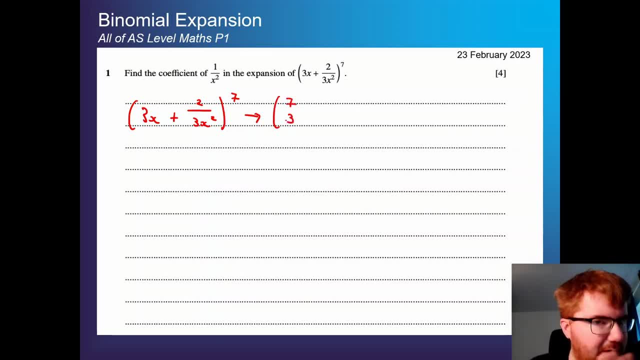 So if I do 7, choose 3,, for example- Which I think is incorrect, but I just want to use this as an example- Then we get this. So this here as 2 over 3x squared to the power of 3, because these need to match this one and this one, and then this one here is 3x to the power of 4.. 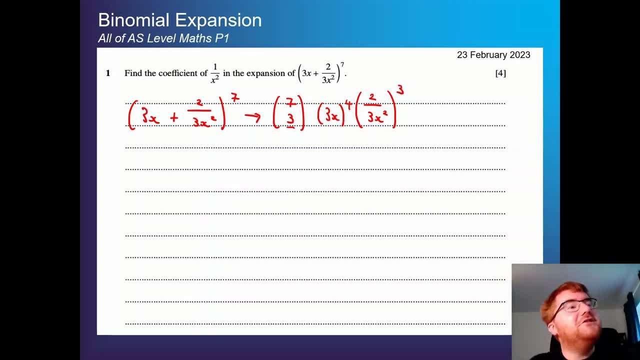 Actually, I think it actually does work. Again, I'm not just choosing the random answer here. I just want to show you the thought process. If we look at the powers here, this gives you x to the power of 4. This here gives you well x squared in the bottom.